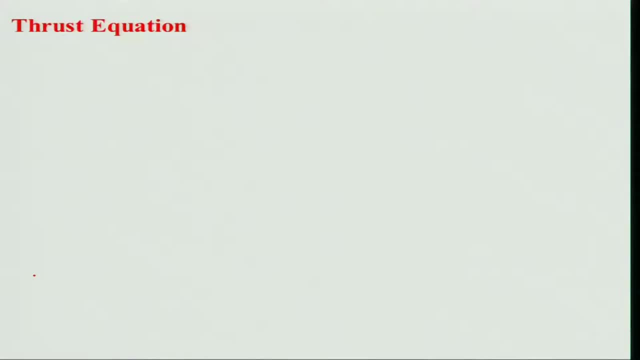 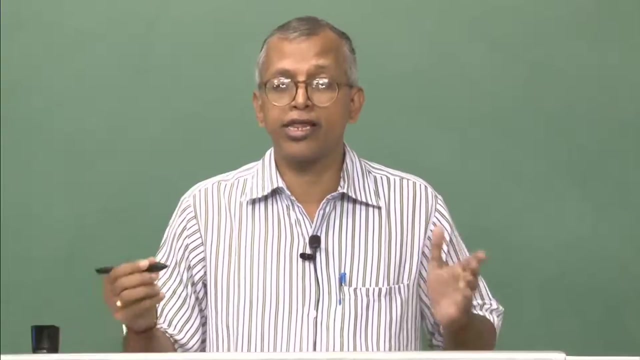 and the other performance parameters. So let us derive an expression for a air, you know thrust pertaining to air breathing engines, And here I have considered a pod mounted engine. I mean, we are not worried about what it contains. what are the components? We know that air breathing engine will be. 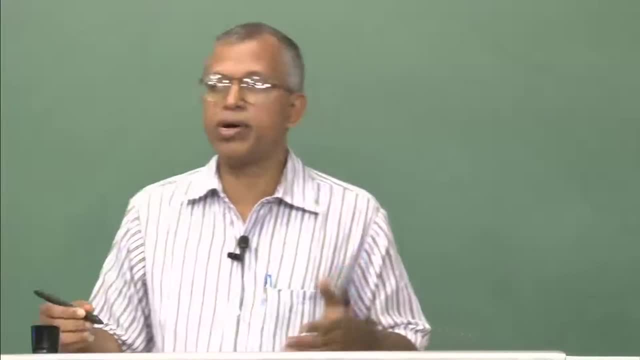 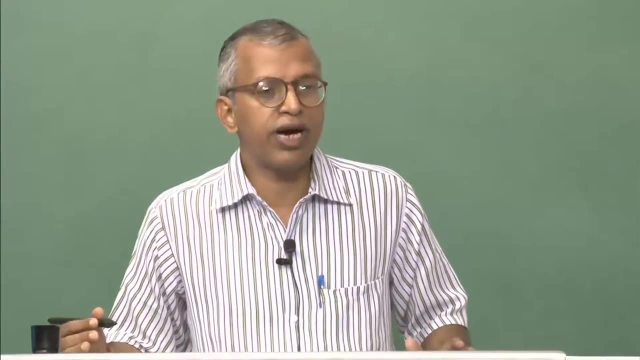 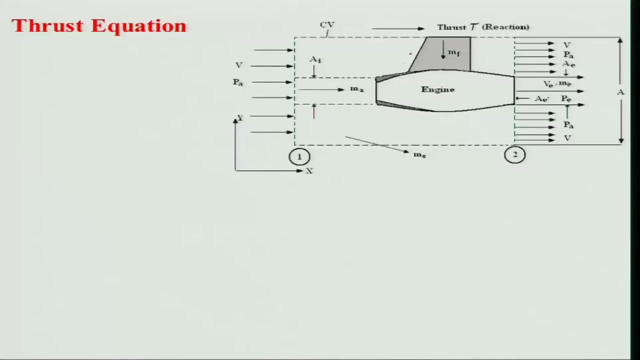 a various component like air intake, compressor, combustion chamber, turbine and nozzle, We are not worried about. We are saying that it is basically a propulsive device or a engine or a propulsive duct and which is mounted in a pod. That means you know there are various. 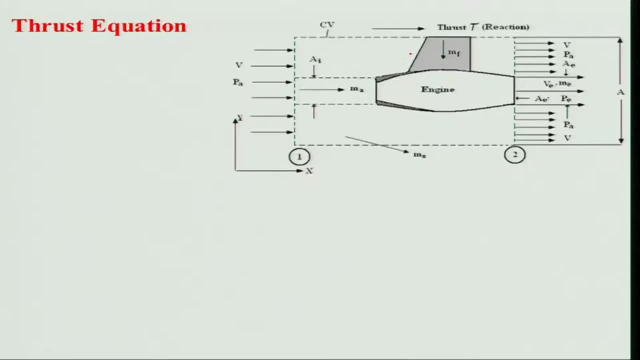 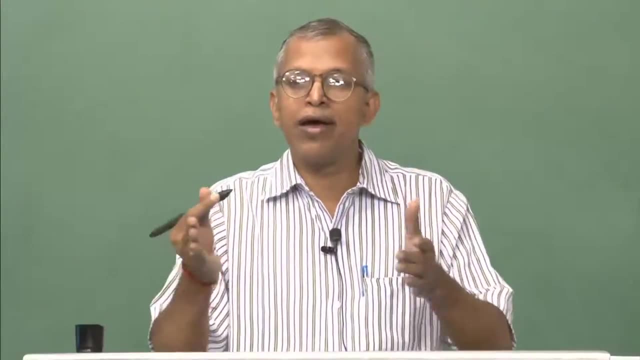 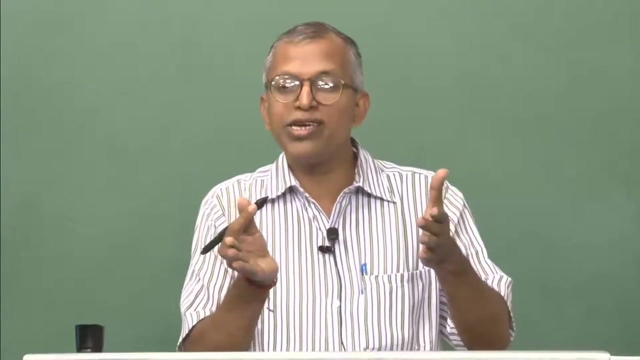 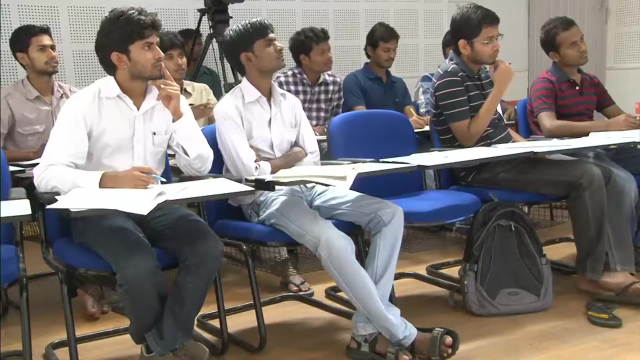 ways the engine can be mounted to an aircraft. right, You might have seen, engines are hanging from the wing and it is, you know, mounted nearby the fuselage right. And in fighter aircraft it will be Engine where it will be located. Where it will be located, but on the front. 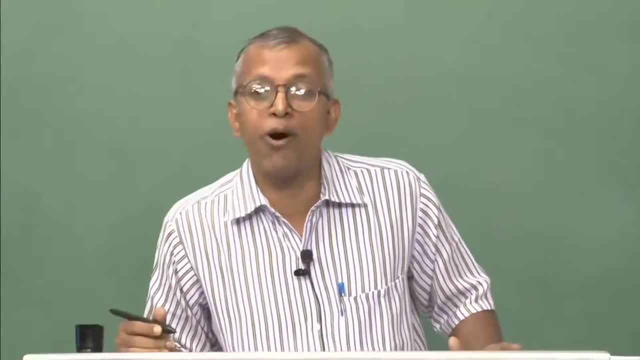 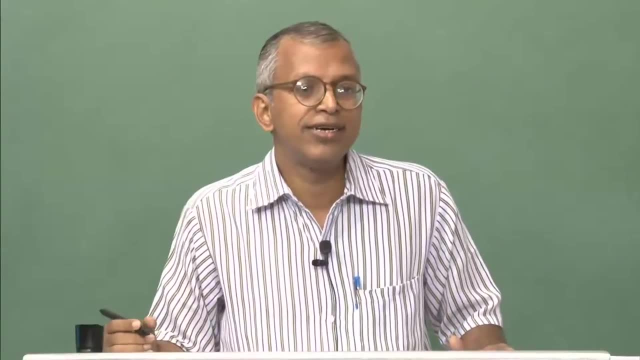 side right, So the air intake will go. So there are various ways of mounting engines, but here we are looking at general. what we look at basically pod mounted engines, right And it is hanging right From the wing, and keep in mind that the fuel flow rate will. 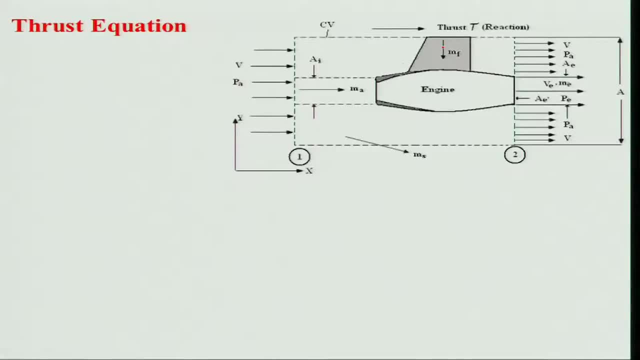 be enteringPUBG through that engines I have shown here and through. this is the inlet of this thing and this is your exit of the engine. That means some air will be entering in and it is going out and of course you will have to add some fuel, combustion will be taking place and then 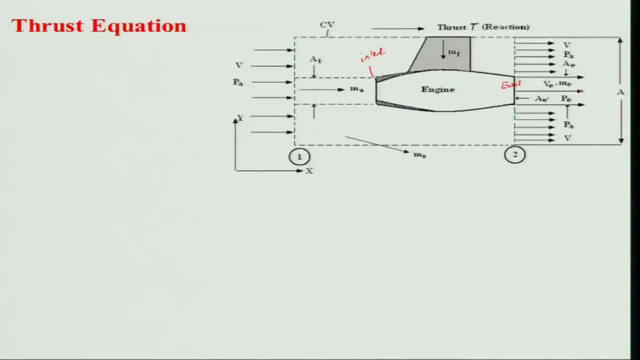 you will add, basically, energy. You will be giving energy so that you can get the thrust. Now, when is air is entering? and what is happening here? It is going at a very high velocity. Suppose it is entering with a, you know v, and then it is leaving with a velocity of v, which 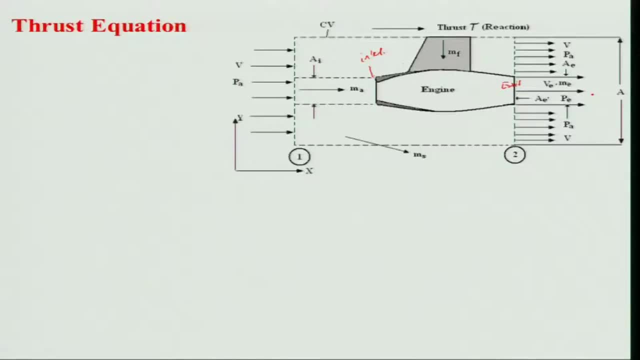 is higher. Why it is so? Because you have added energy into it and you are trying to accelerate the exit velocity and keep in mind that we have done some approximation here. Is it that It will be coming through that way? that, whatever vectors I have shown, Of course it will be? 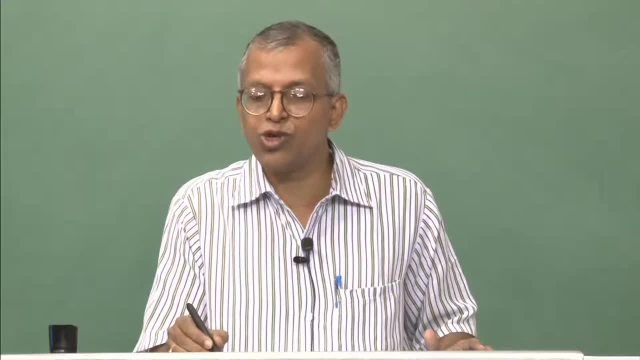 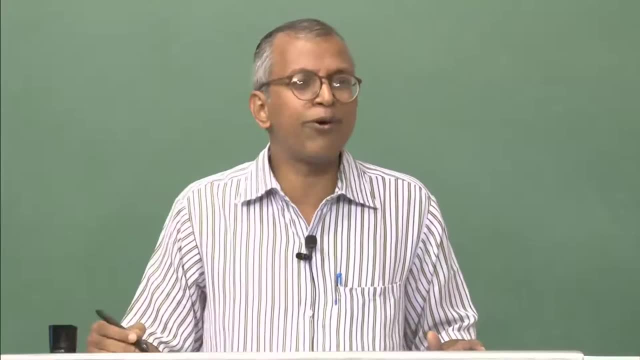 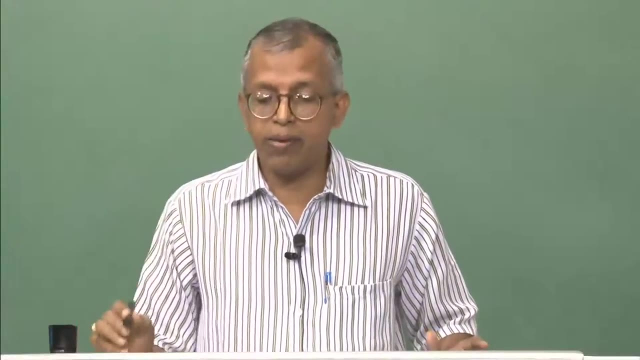 true, provided I assume that is one dimensional proof. In real situation there will be boundary layer, There will be some swelling, you know, because from turbine it is coming. So there will all those things we are not considering. Please keep this in mind. and now, if I want, 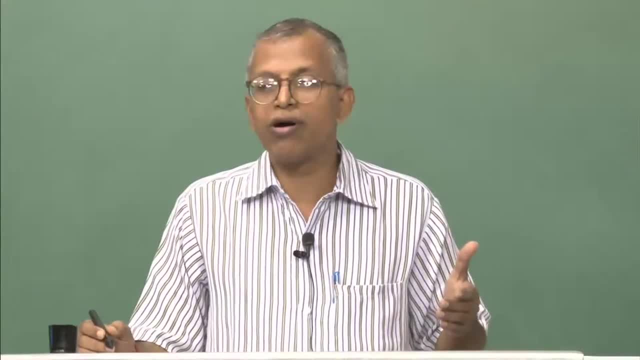 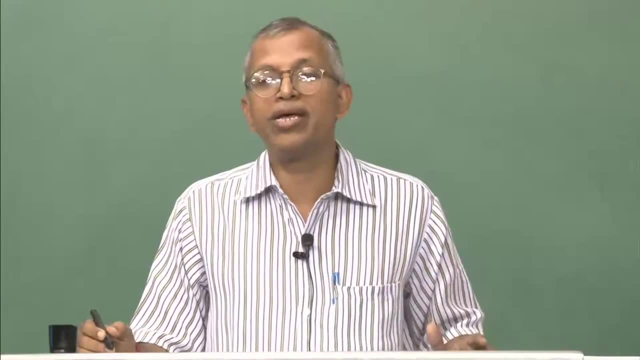 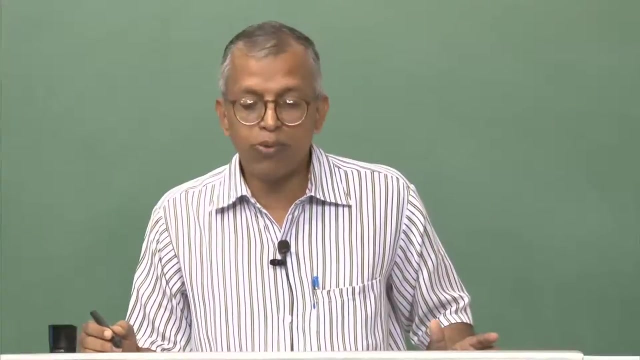 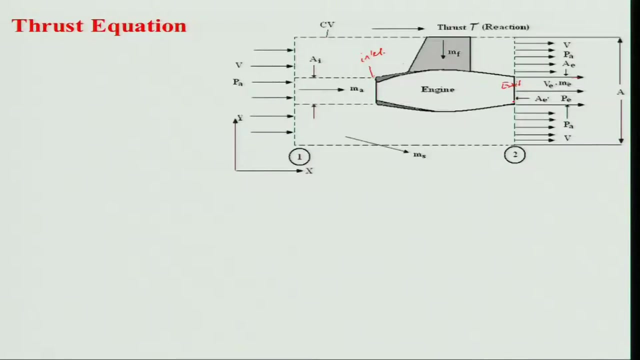 to find out this thrust equation, I need to invoke the Mass conservation equation, momentum conservation equation. For that I need to place the control volume Where to control volume? When to where to place this control volume is important, Of course. here it is very. I have shown here, but why I will put like this, For example: 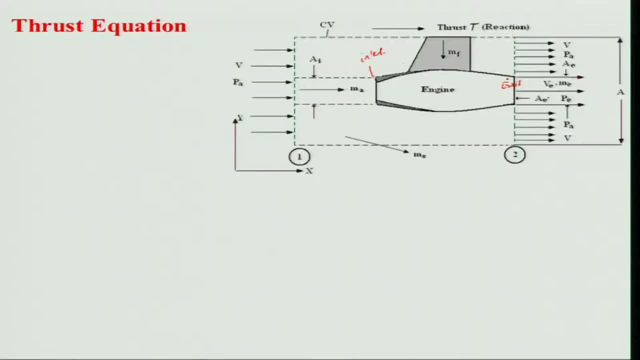 why my control volume will be just exactly at the exit of the engine. Why not? it is far away. The control surface bottom- sorry bottom- and the top control surface is away from the engine. Why not nearby or just here itself? And similarly, why my this left hand control surface, you know, 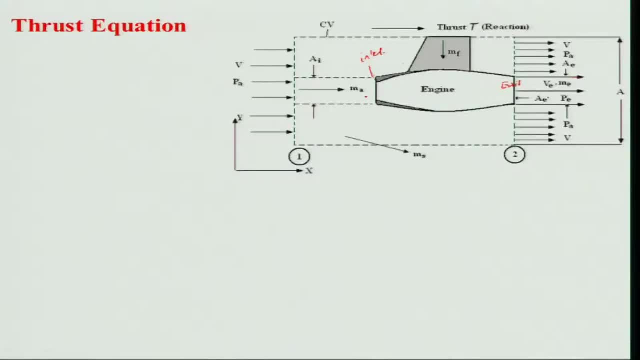 why it is in this place, far away from the inlet. What is the reason? I can place control volume anywhere, Is it not? Can I not put it here somewhere? Or can I not take this as a control volume and then do that? I can do Yes or no, But 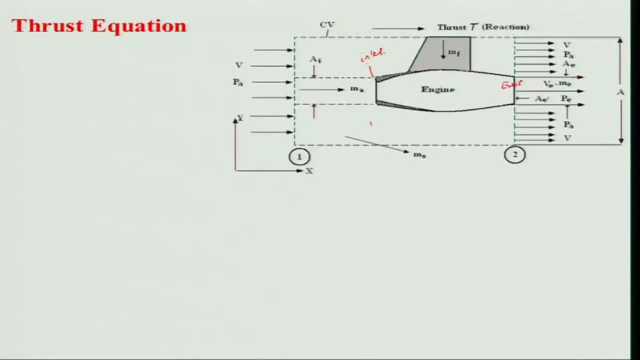 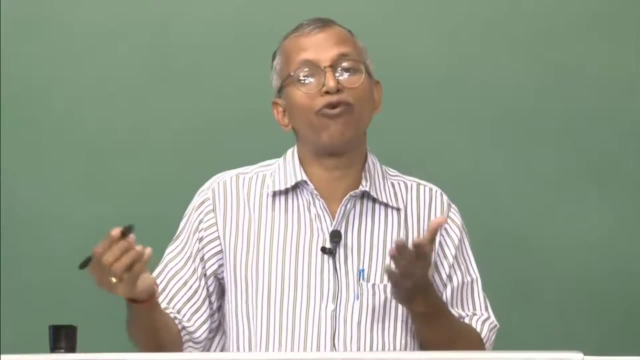 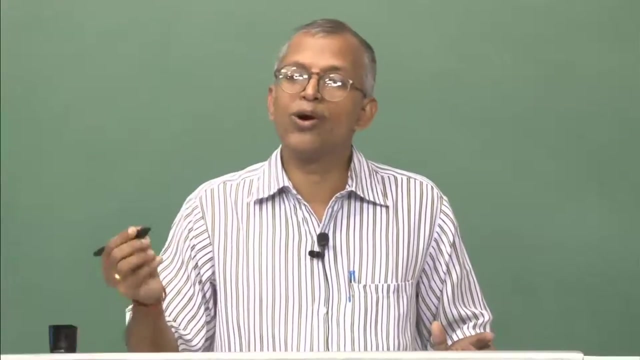 if you do that may be analysis will be quite complex To have a simplified. we have done that and keeping in the one dimensional flow in mind, Because if I use two dimensional it will be little complex to do that. that is the only thing, and keep in mind that we. 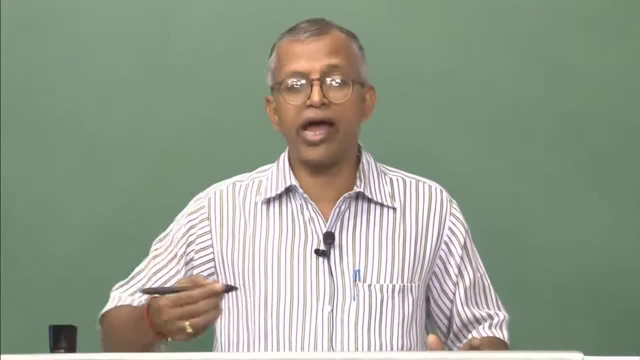 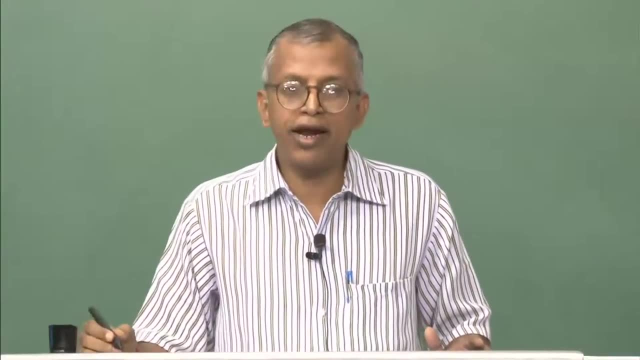 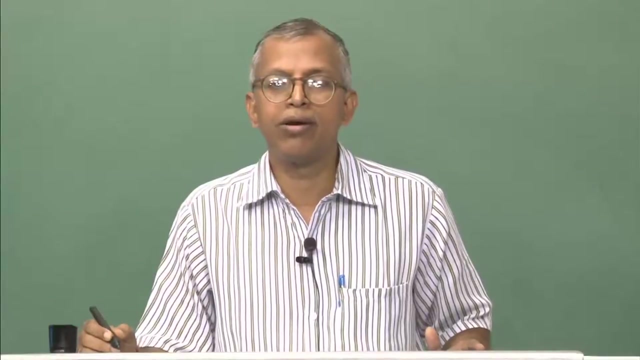 are not considering the unsteadiness. that means it is not, like you know, taking a somersault by an what you call fighter aircraft, which is be unsteady. It is a label flight what we are considering to deriving this thrust. Therefore, we are considering the aircraft. 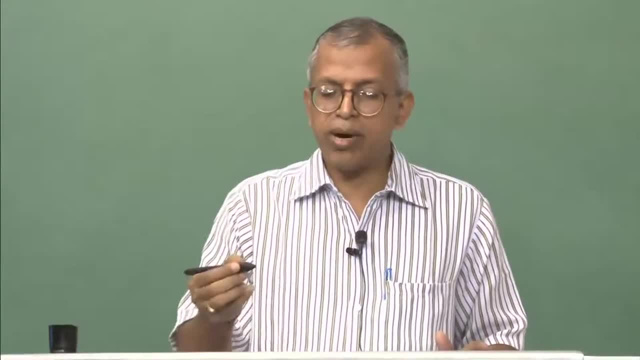 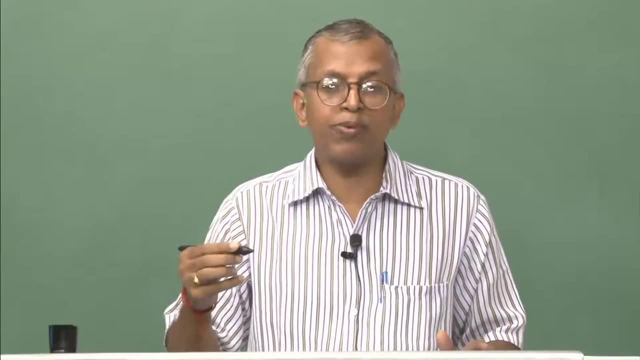 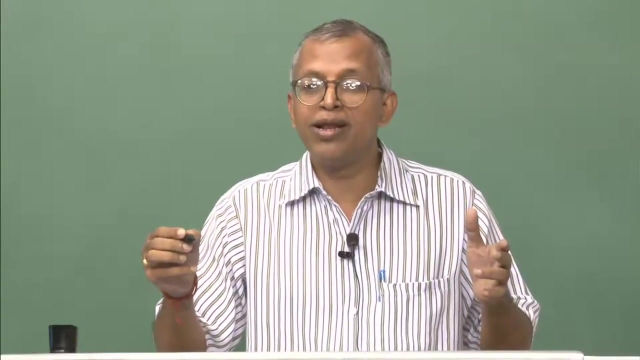 that is moving steadily and some other assumption we will be doing. but as you go along you can note down the assumptions, but I would not be stating, as I had done earlier. like you know, steady flow process irreversible. There is no frictional effect or Eulerian. 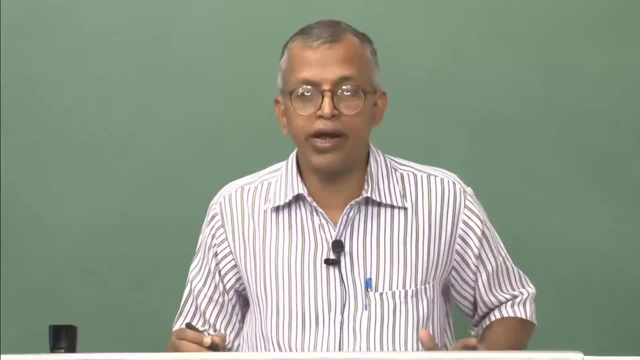 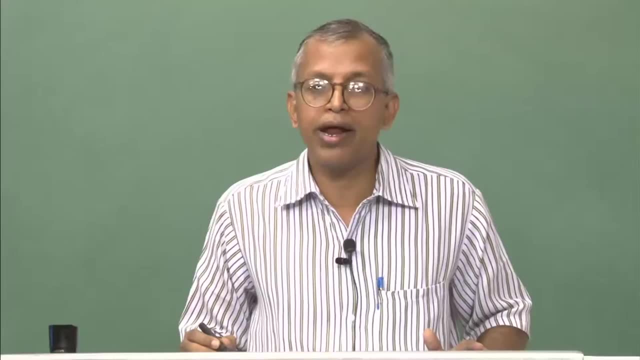 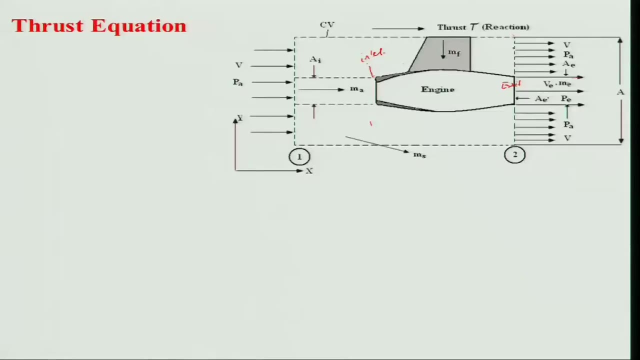 flow, all those things I am not stating in a very systematic way, but as I go along, I will tell it Some of the things I would not be stating very explicitly. So why I am placing this control surface here? because, as I told you here, I can assume the flow to be one dimensional. 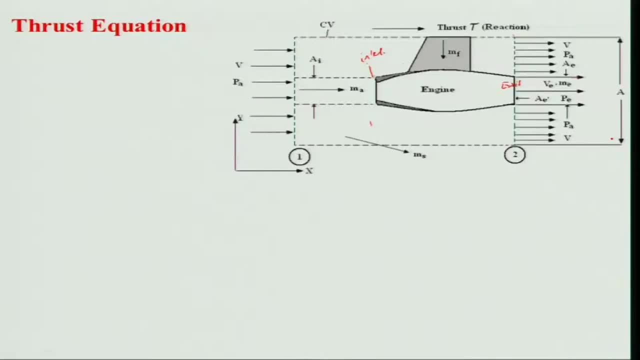 but if I place somewhere here in this zone, then can I place, do that. if I do that, then the flow will be two dimensional nature. It is a jet flow- entrainment will be there and the flow it is a wake region. So therefore, 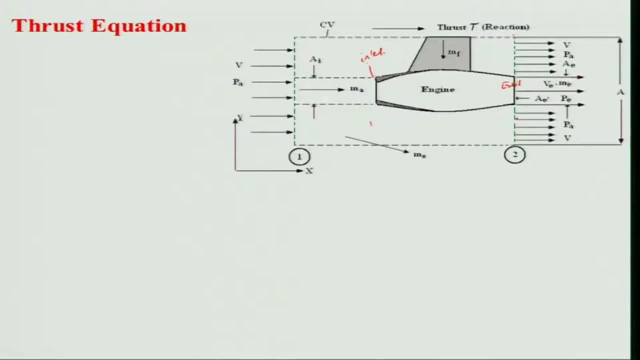 it will be difficult to talk about. So therefore I will put it here where I can assume the flow to be uniform at the exit and also the other portion from here to there. it will be uniform And we are assuming that it is. this flow is coming with the same velocity, with 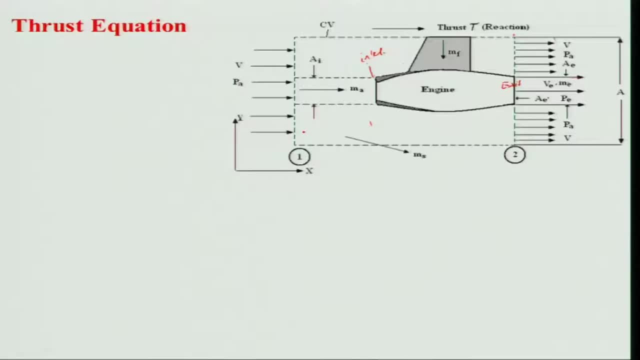 which it is entering the control volume. at the inlet, that is the station 1.. And at the exit, I am saying station 2 and keep in mind that this surface is far away, because the effect of, because if I take a stream line over here, what will happen? it will be taking. 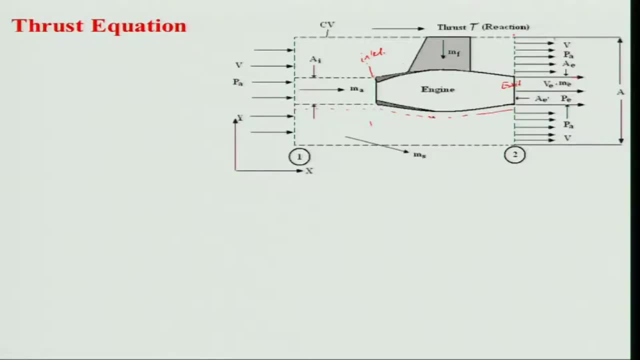 the shape of the things. And then I am having two dimensional flow. if I take this, resolve it: one in x direction, other is in the y direction. So therefore it will be two dimensional. if I over here I will be not considering, I will just say that this y dimension, some flow will be coming out because there is obstruction. 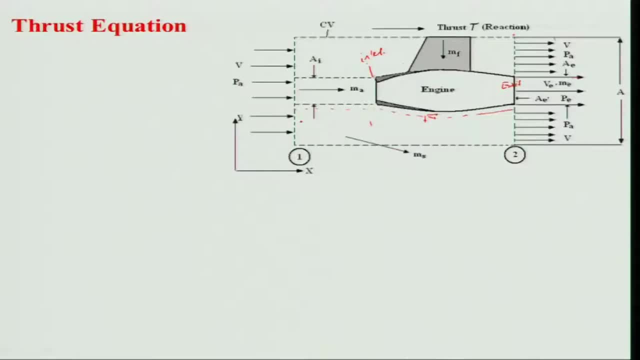 but that will be negligible. we will see that. And it is placed here So that the flow can be taken uniform and I am not worried about how much it is, because if you know that actual flow will be little diverging in this zone in the inlet, because the inviscid flow will. 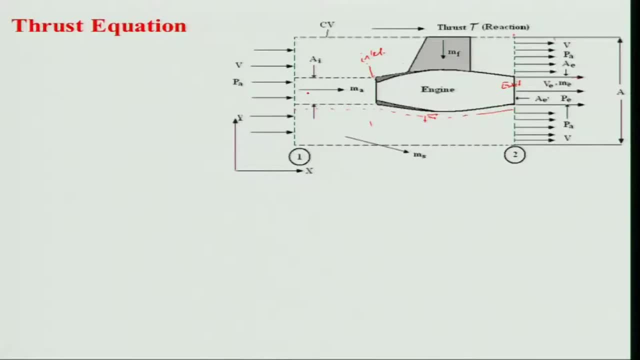 be there And you know it will be diverging towards that. So let us now look at considering steady flow process. the continuity equation becomes what you call rho v, dot, n, d, n, And if I take for this control volume, sorry, first we will. 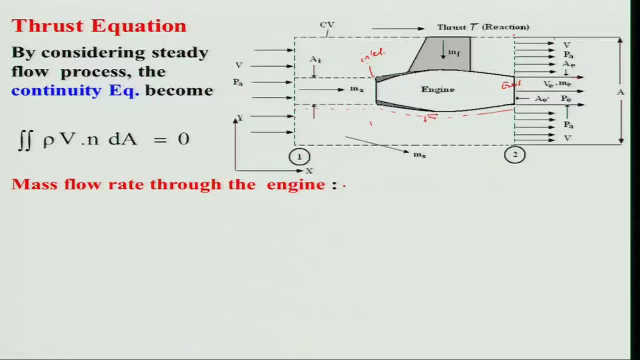 take the mass flow rate through the engine. If you look at what is the mass flow rate it is entering, if A i is my this area, Then I can write down that how much mass is going out from the engine. that is rho, e, v, e and this is my area. what you call A, e, right I? 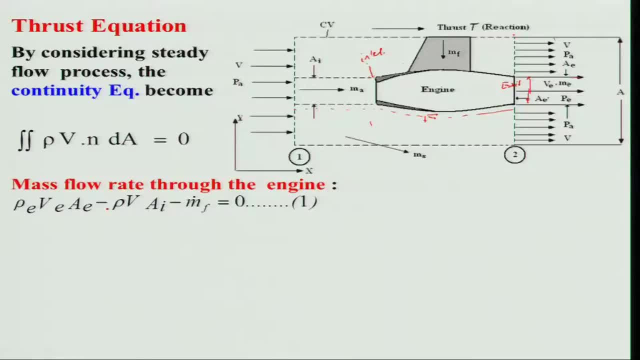 have shown here: A e, So rho e v e, A e minus rho v, because it is entering with the rho and velocity v, with this And rho v A i. A- i is the capture area, what I call- and minus m dot f because some of the fuel is entering. right, Because whatever the fuel is entering, 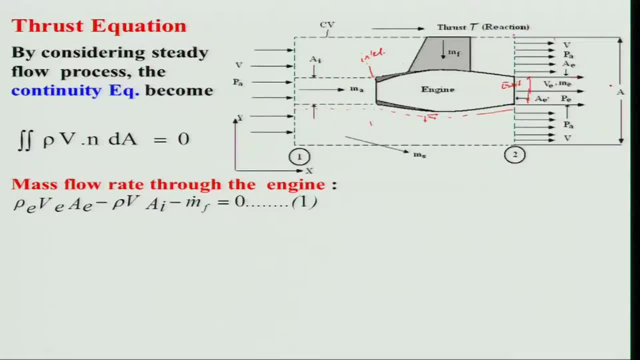 whatever the mass is entering, you will be going out of this. right mass is conjured. that is the exit mass flow rate. So if I want to write down in a mass form I can say mass flow rate of exit. this is basically if you look at m dot e and this is your m dot i, and 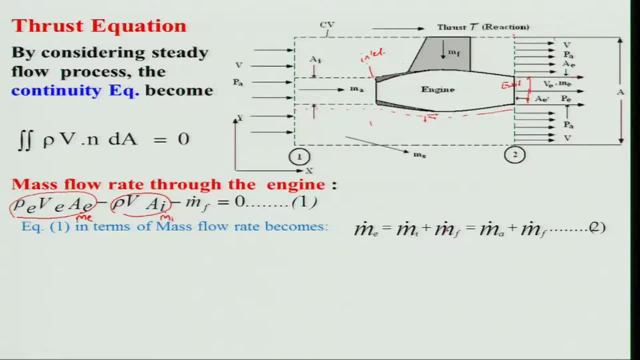 this is m dot f. That means m dot e is equal to m dot i plus m dot f. you can say this is basically, I can say that right. that means how much mass flow rate of air is entering into the engine. So now we will be invoking the continuity equation for the entire control volume. what? 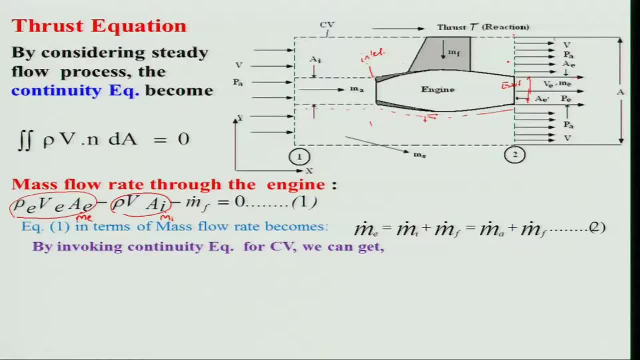 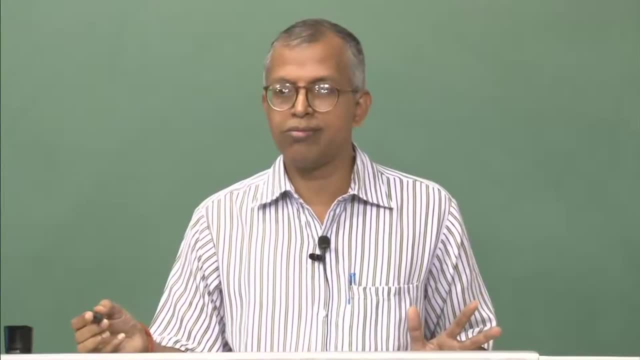 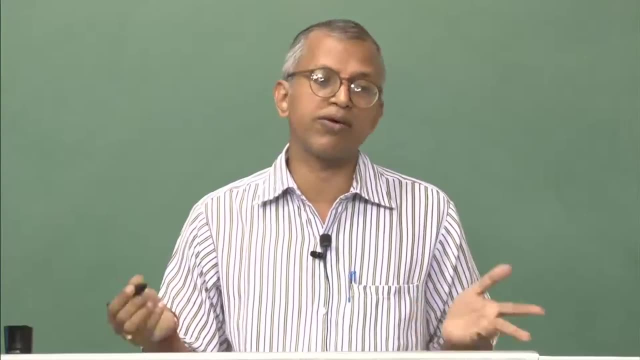 we have done till now. we are considering the mass conservation for the engine. That means how much mass is entering, how much mass is going out, and that is the mass leaving the engine is equal to mass of the air entering into the engine, plus mass of the fuel is a. 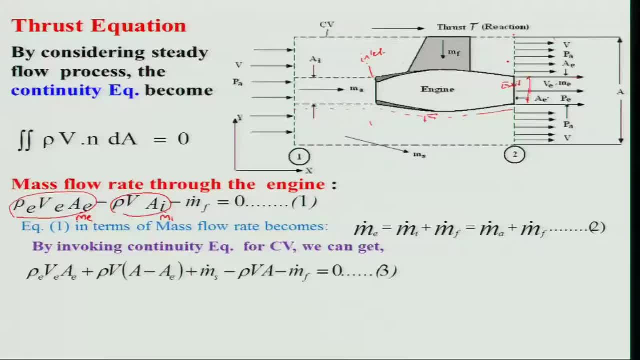 very simple one Now. what I will do, like we will be considering in this domain, that is, you know, and how much is going out here and how much going at the exit. So if you look at how much is going at the exit, that is rho e in this from the engine, rho e v e A e right and in this region. 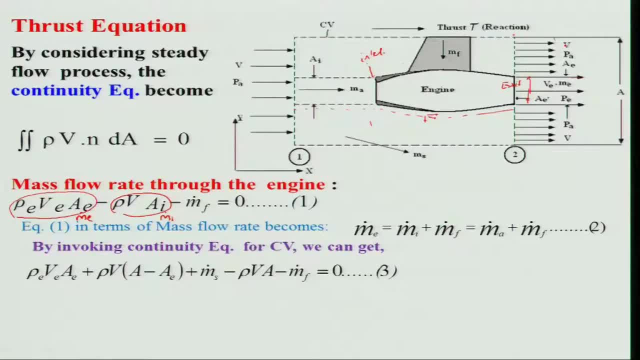 what you are doing, like that is, is coming Coming to the same velocity. this, again an assumption, because near by it would not be because of stream line it will be having different values. but however, we are assuming that v, So that is rho v, into area. what is that area? total area from here to here of the control. 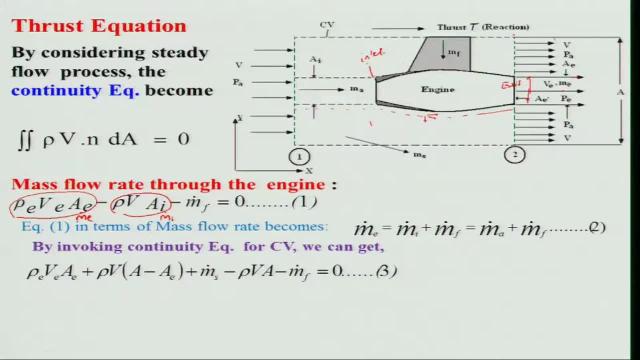 volume, are it cross sectional area A and the exit area A, e. So therefore this portion, you know, if you look at this portion, is nothing but A minus A e, right? So when you Look at this portion, So are you people are getting or not, For example, I can say that like, this is my a. 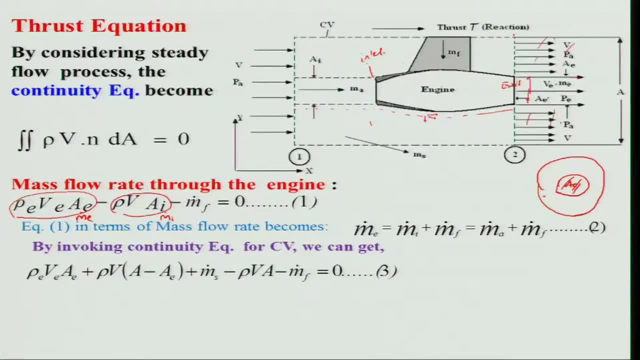 this is the ae and this is what you call. this is basically a. So what? this area is nothing but a minus ae. that is the through which this is coming. So rho v v, a minus ae plus m dot s, and m dot s will be coming like this: in the y direction- sorry, x direction. this. 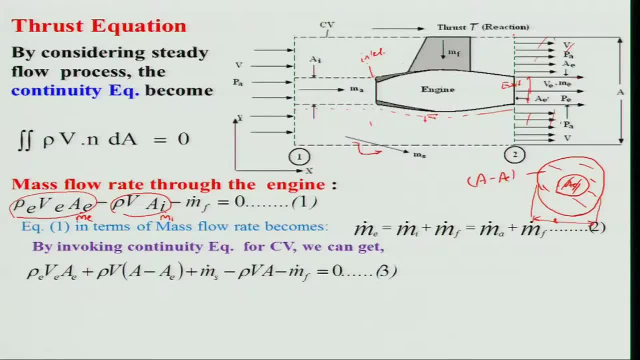 is the x direction. We are assuming that y direction will be very, very low as you go away. you know that kind of thing, whatever that. but that is not true. it is an assumption. So some component will be there then clubbing this, what you call clubbing this equation. 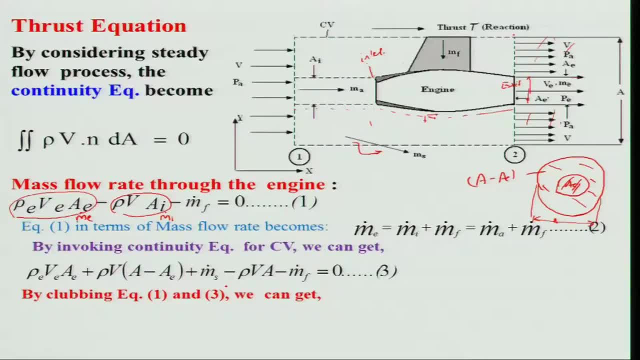 one and equation three we can get, because we are interested to find out what is m dot. So I can write down: m dot s is equal to rho e v e ae plus rho v a minus ae right Plus rho v a plus m dot f, because I am taking this left hand side, then I am getting that. 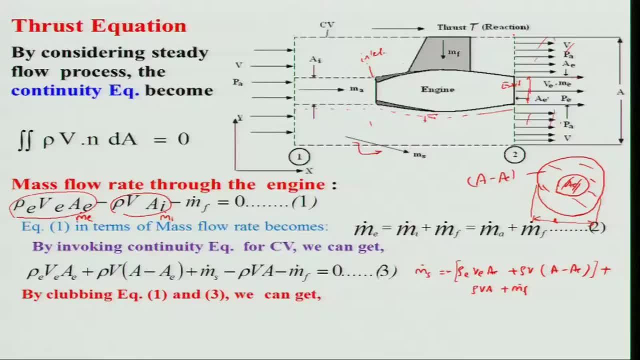 and what I will be doing. in place of this m f, I will be writing rho e v e ae. that means, in place of this or in place of. I will be writing, basically, Now, what we will do. we will just put this: in place of m dot f, we will, you know, use this. 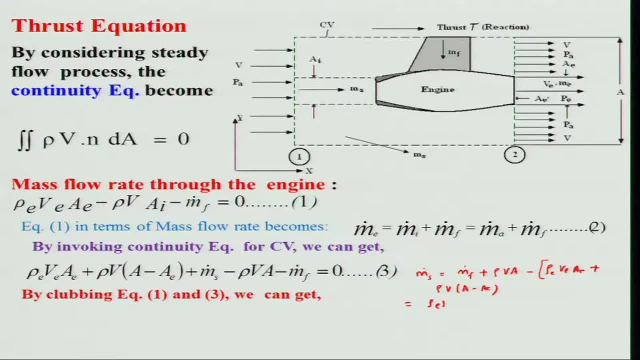 equation, one that is nothing but rho e v e ae minus rho v ai, and the same thing as rho e v e plus rho v a minus ae. Keep in mind that I have left one term here, so I will add it: rho v a. 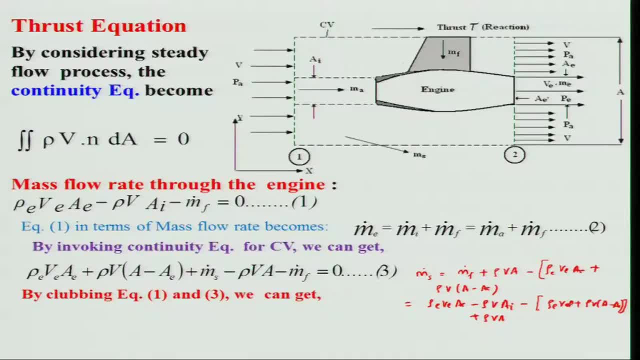 So if I cancel it out, this term will go away and similarly, this term will go away with this term. right? So what I will get, I will. if I simplify, I will get m dot s is equal to rho v ae minus ai, and if you look at I will get m dot s is basically I can get. 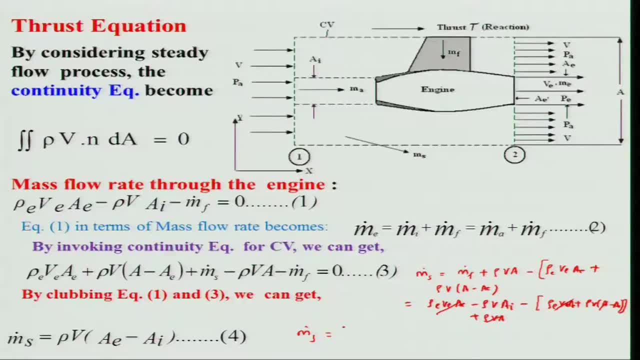 rho v ae minus ai. So this will be rho into what you call ae minus ai. that means this is the amount of mass flux which will be going through this control surface, right and the down. of course, up like it will be going out because there is a body. 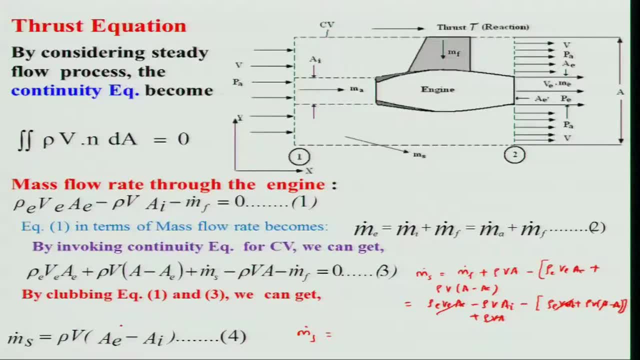 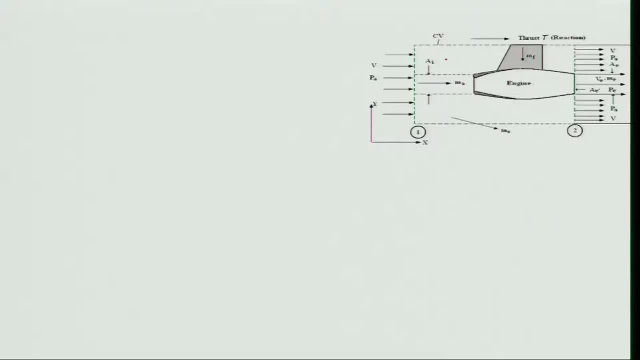 We will be using this and find out a expression for a thrust So that if you look at the first wise keep in mind that this thrust is actually acting over in this direction. but when we take this from the cut, from the what you call part, then the reaction to thrust 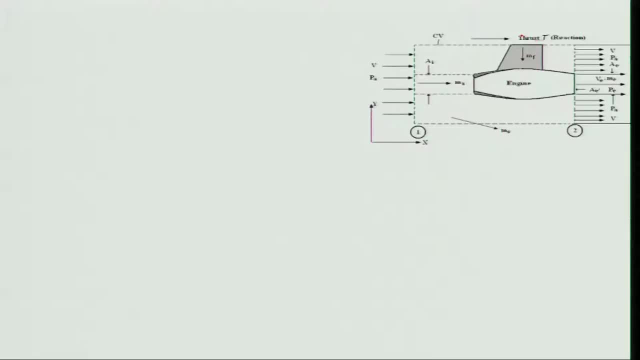 will be in this direction, right. So now what we will do? we will be using this momentum equation And we are neglecting the body force right, which is will be very, very small to be neglected, And we are considering momentum equation. 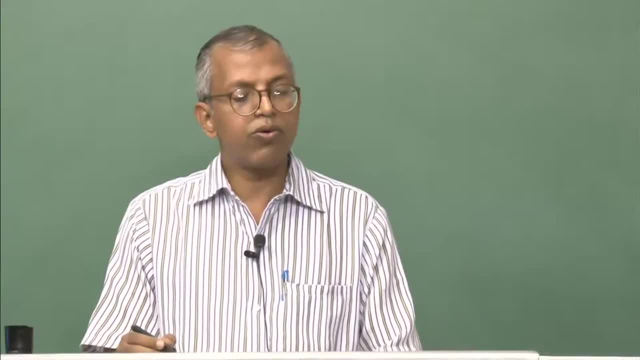 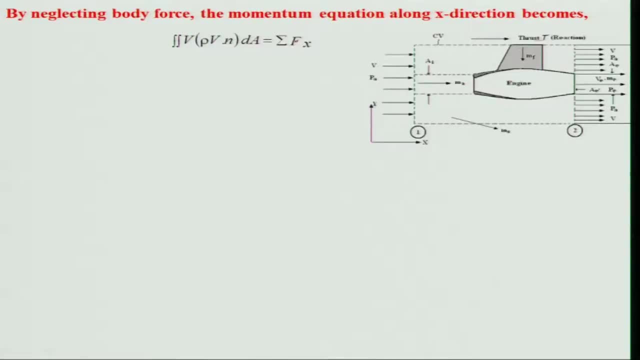 along the x direction only. So when we will do that for a steady cases, we will say this total flux is equal to some momentum flux is equal to summation of the f, x, a force along the x direction. So what are the forces acting on the x direction? One is the thrust: 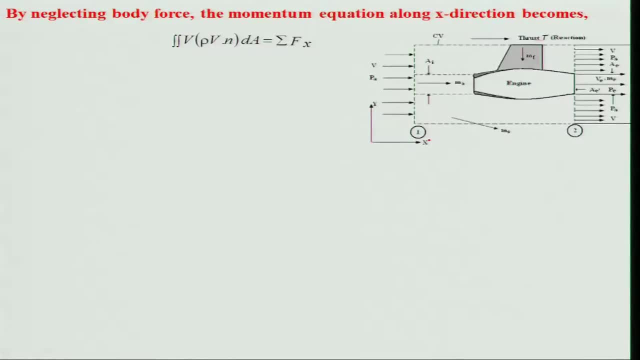 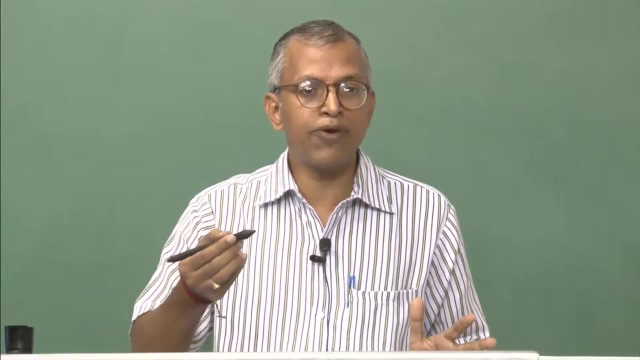 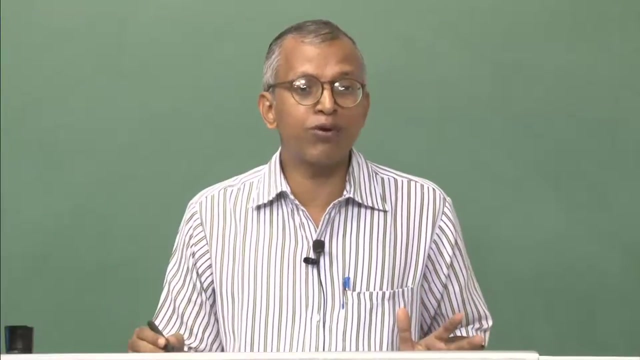 which is along the x direction. and what are the other forces are acting? Drag: we are not considering. It is a level right thrust is equal to the drag. Am I right or wrong? So what else other force will be acting on the control volume because we are using a control? 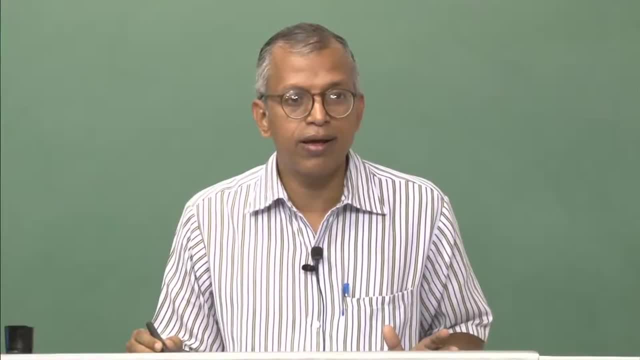 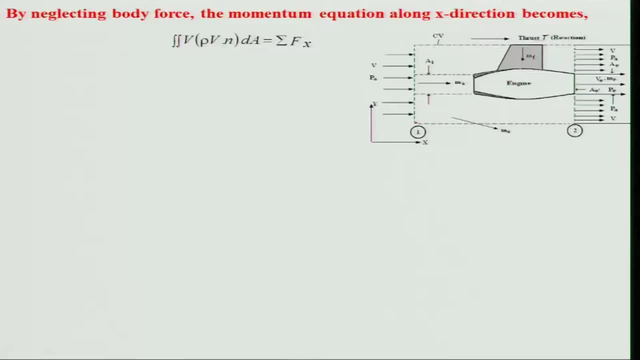 volume. What are the other forces will be acting? It is a pressure force. So what will be pressure force in the, this surface? This will be what you call, Like p into a, a whole surface and same cross sectional area. Similarly, what will be pressure? 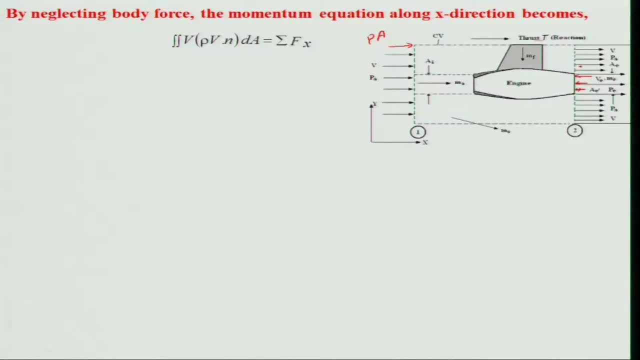 force which will be acting here in the exit. That will be p, e and a, e and whatever this annulus area leaving this exit portion, if you take it as a circular. So what will be there? That will be the pressure force. 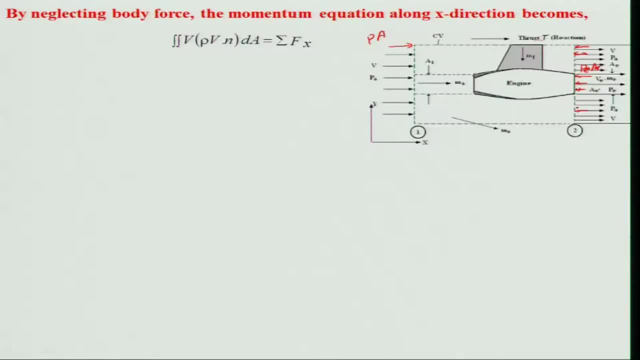 Pressure force which will be acting over in the opposite direction, to that which will be p, a, a minus a e, which will be opposite to the x direction in this way, So then we can write down that the thrust force or the summation of the force along the x is thrust. 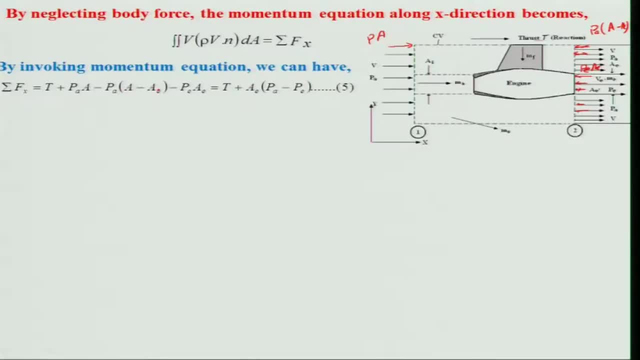 plus p a a, minus p a a minus e And minus p e a e. So if you simplify this, what will you say? This will be cancelling it out with this. So you will get t plus a e, p minus p e. Now we will be evaluating. 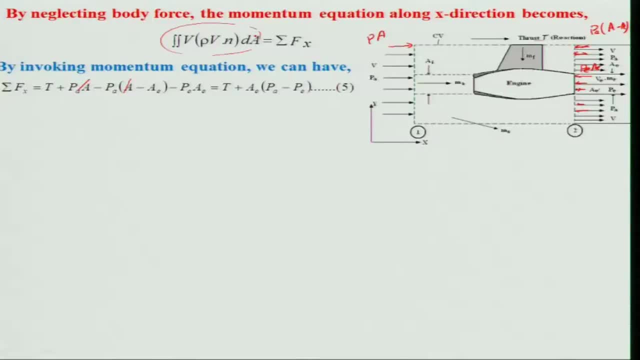 this term like momentum flux term for this control volume. So you will do that. Then what I am getting? I am getting m dot e v e plus p e a e plus p e a e, minus p e a e. 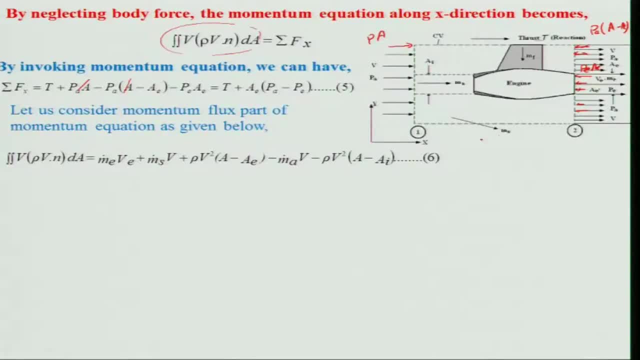 I am getting m dot e v e plus m dot s. This is the mass flow rate and which will be moving with a velocity v because it is far away. So it will be moving this fluid along the x direction. That is an assumption, because we are assuming along the y direction, that 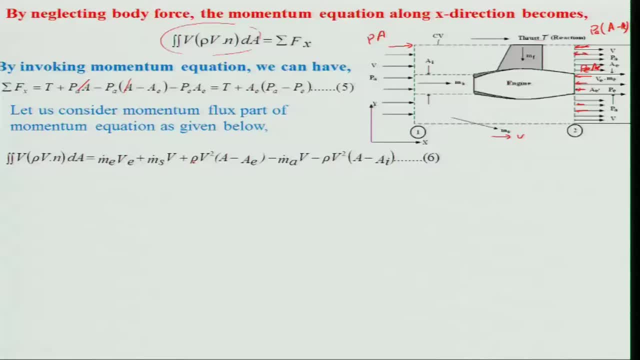 mass flux is negligibly small. Plus rho v square a minus a e. That means this amount of which will be there because we are considering in the exit. and what about this? This is also rho v square a minus a e. This term minus what is the inlet? Inlet will be m dot a v. 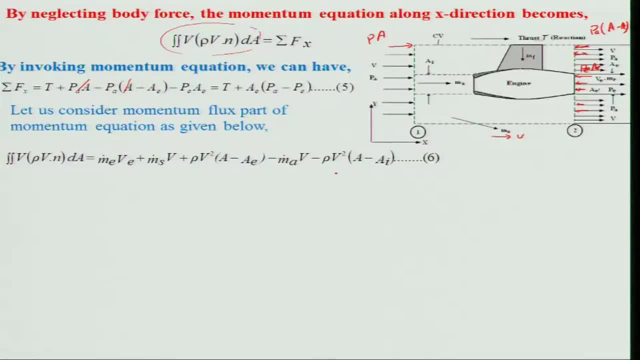 in this region minus rho v square a minus a i, because if you look at, you know this, this amount is entering into m dot a into v, but in this annulus region it will be rho v square a minus a i, because this is a. i Keep in mind that a i need not to be same. 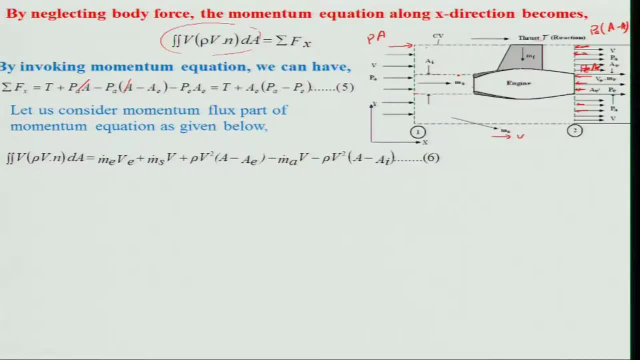 as a e. It may be same, It may not be. So if I now put this equation 4 into this place and simplify, So you know it will cancel it out. I will get m dot e v e minus m dot a v, And when: 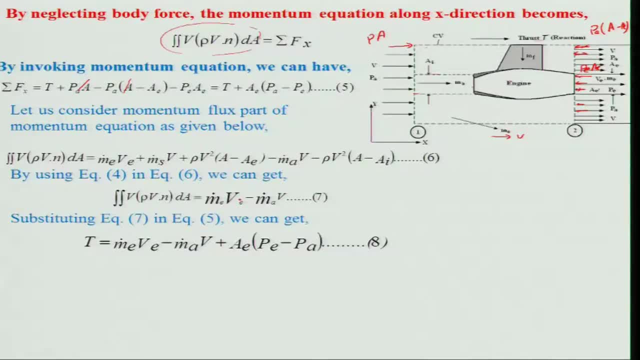 we substitute this expression, you know, over here this is basically equation or equation 5, like this I will get: thrust is equal to m dot e v e minus m dot a v plus a e, p e minus p a. So if you look at, this is the expression for the thrust And what you could see There. 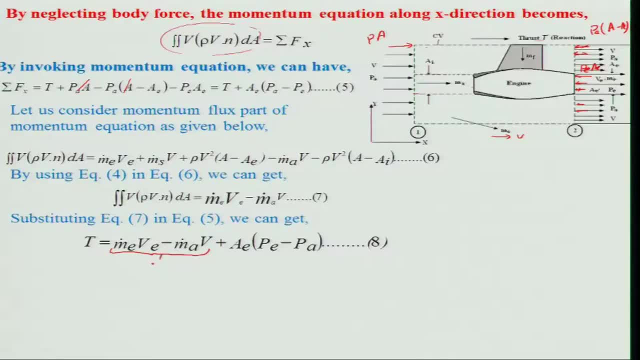 are. this is basically momentum thrust. And what is this? This is your pressure thrust And if you look at, this is basically is the exit, This portion is your exit thrust And this is what This is inlet drag. right, That is inlet drag, because that is a acting 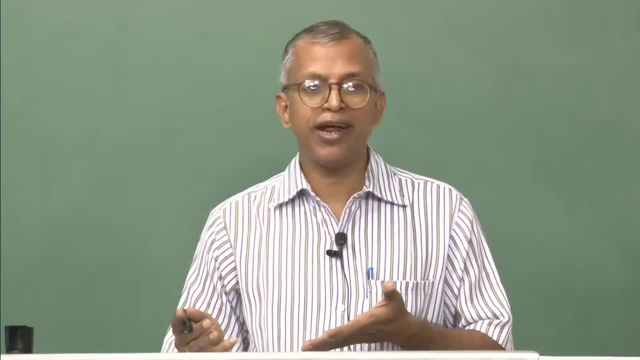 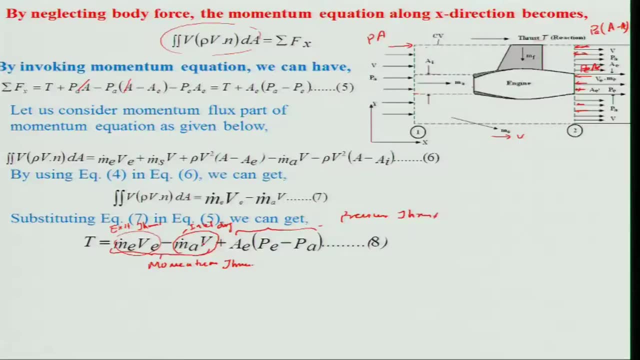 you know, like whatever thrust being produced by the jet, right, It is being acting, So it is being swallowed by this inlet drag, And one has to reduce it as much as possible, right, Then what we will gain. If my velocity, the flight velocity, is 0,, then what I will. 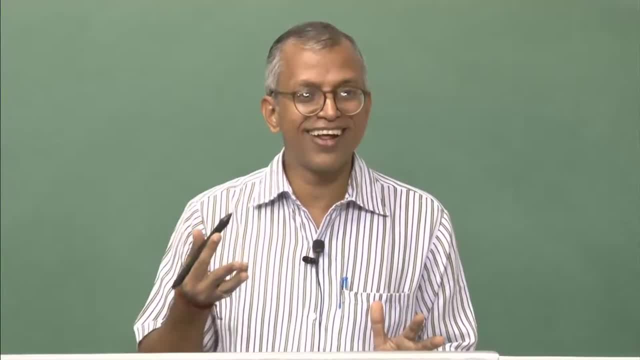 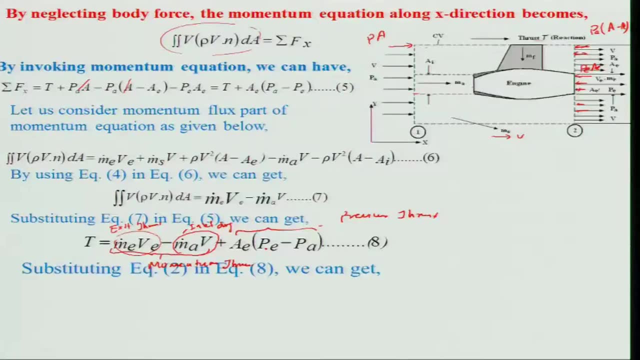 do. I will be only on the land, right. But I may get a thrust And keep in mind that this thrust can be maximum values, right, And this thrust can be maximum when it is fully expanded. That means if the nozzle is fully expanded, that is p, e is equal to. 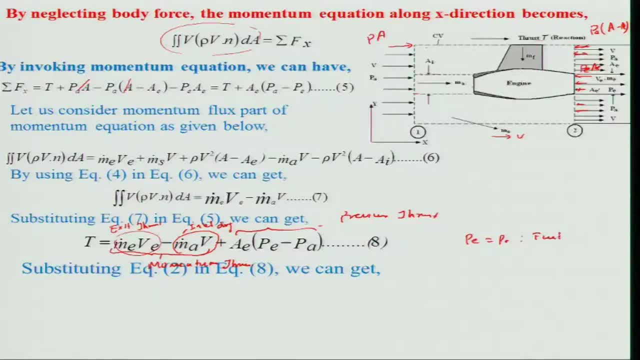 p a That is fully expanded nozzle right. Then you will get the maximum thrust. Now what we will do: This: we will now substitute for m dot e, because we know what is m dot e. m dot e is equal to m dot a plus m dot f right That we have already derived When 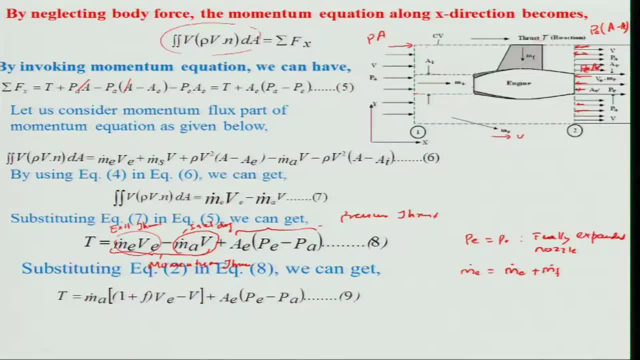 we substitute these values I will get. thrust is basically m dot a plus, you know, 1 plus f, v e minus v plus a, e, p e minus p a. How I am doing that? Because you know, like f is basically m dot, f by m dot. 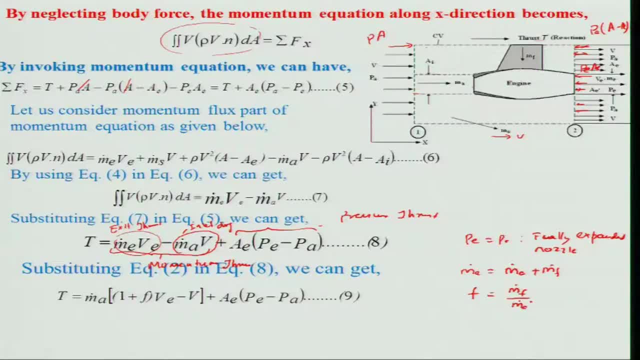 This is the fuel: a ratio by mass right In place of m e. I am putting, I am taking the m dot a out, So I am getting that. Keep in mind. this is a very, very small number Generally. 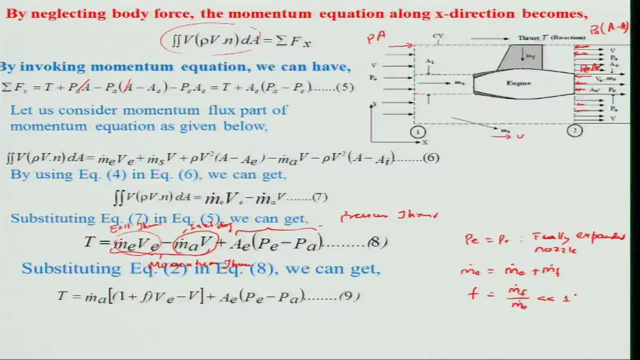 you know it is a very, very less than 1 kind of thing. So sometimes, and rather majority places, we will be neglecting it. right, When we are discussing now, I mean like onwards, several places we will be neglecting, We will say that f is very, very, you know less. 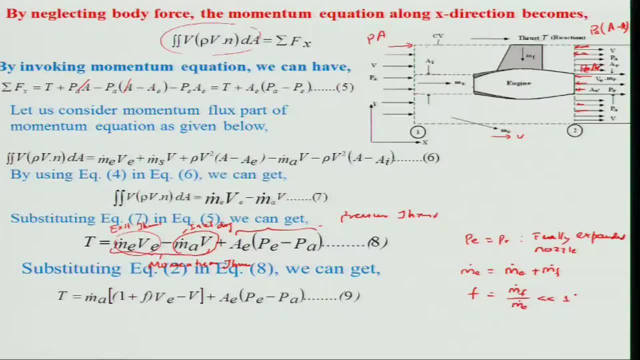 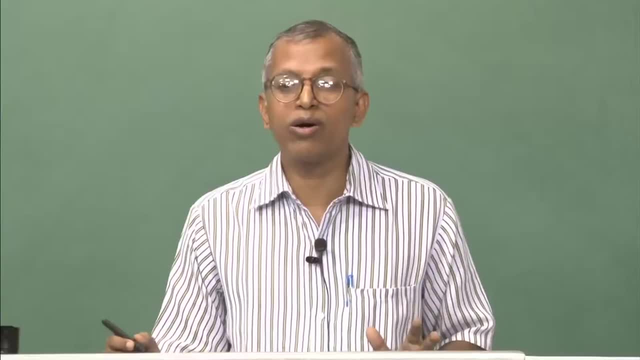 than 1.. Therefore, it will be equal to 1.. What will be the number f? Can anybody tell me what is expected? It will be around 25 is to 1, it can be 30, it can be you know. 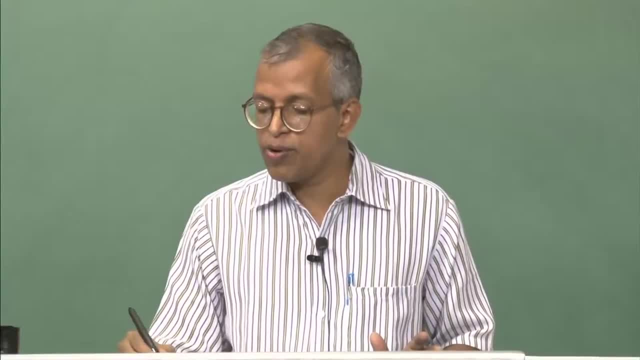 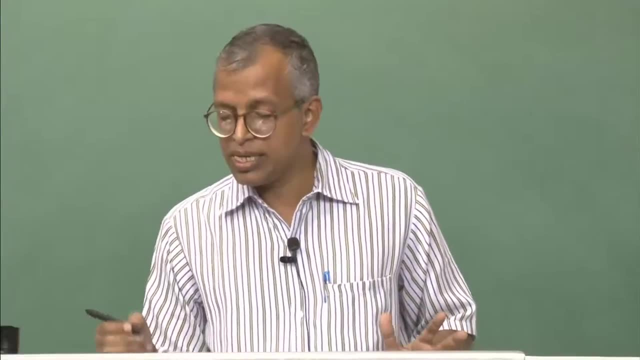 kind of things. right. That means it will be 1 over 25, right or 30. That means it air fuel ratio will be 30 is to 1, like fuel air ratio will be 1 over that. it is a very 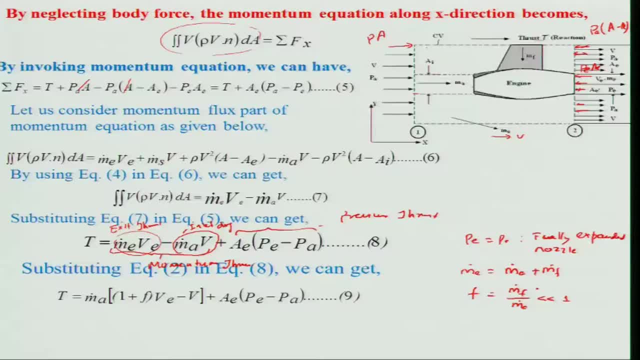 very small number, So we can neglect that and this expression. if I you know, in the case of rocket engine this will be v, will be 0, and then I will get this 0, then I will get a thrust expression as m dot e, v, e plus a, e, p e minus p? n. We will be discussing little. 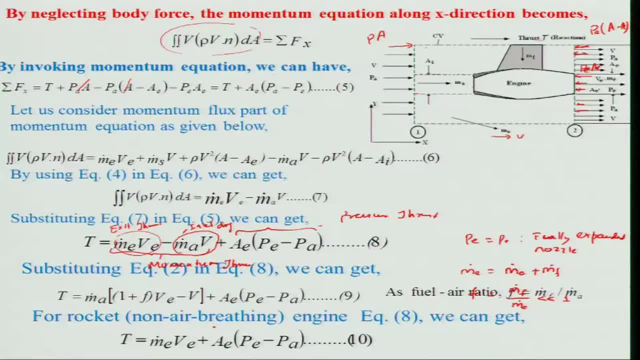 bit more about when we will get into rocket engines may be. I will invoke this expression again and talk about some of the things. So what is the difference between non air breathing and air breathing? only that inlet drag will be there and the expression is similar. Now, 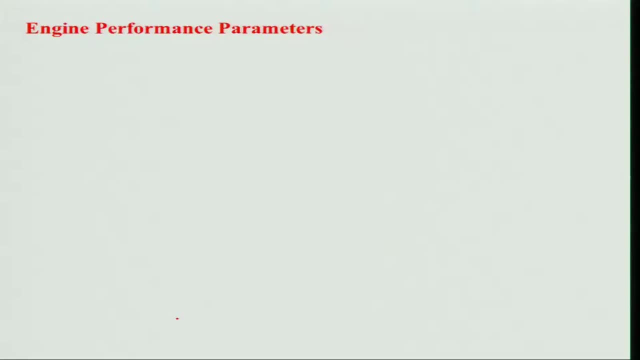 we will be looking at Engine performance parameters. what are those? there are several efficiency will be defining. So first we will discuss about propulsive efficiency. and what is that is basically ratio of thrust power to rate of production of kinetic energy of the exit jet, because you are basically 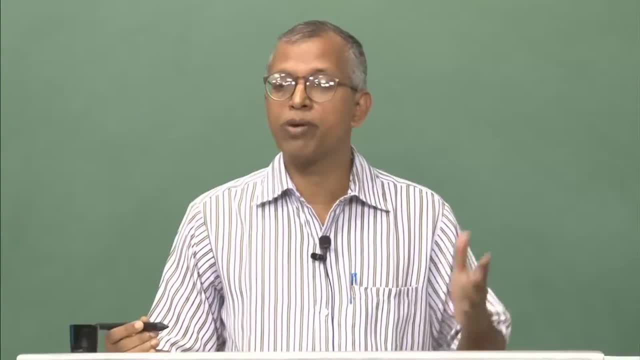 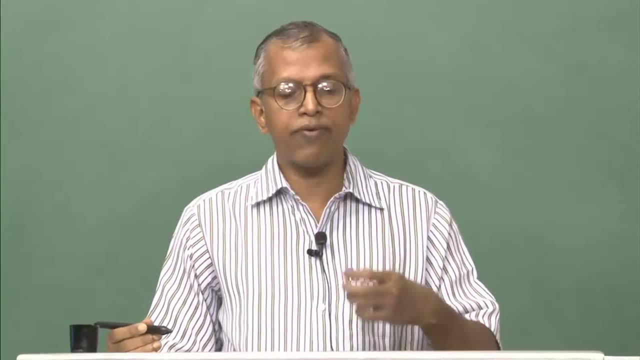 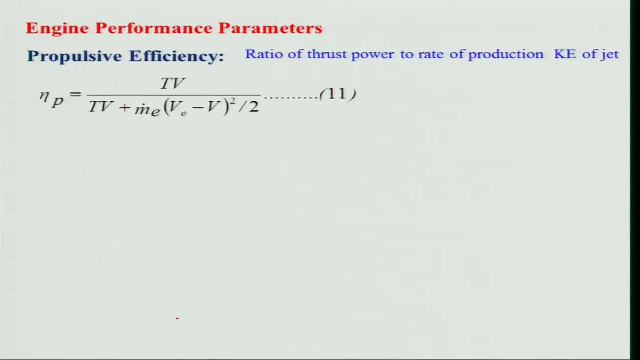 that is why you call it jet engine, you know, or a jet propulsion. in some places people talk about it. we use because the kinetic energy and then from that we will be getting the thrust power is a ratio. So mathematically, if you want to look at, you can write down. 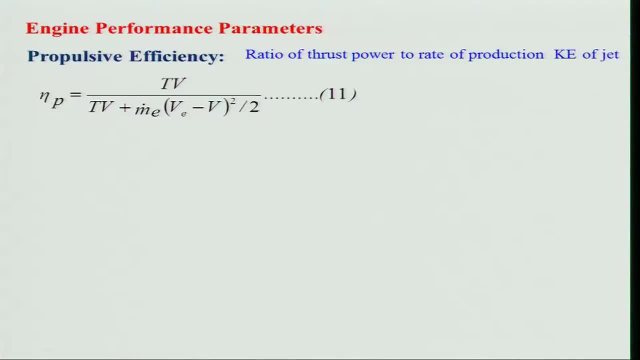 thrust power means thrust into velocity that will give me thrust power. this is nothing but your thrust power and the thrust power plus the amount of energy which is going out in the exit. and keep in mind that this is what this portion is: the, you know, kinetic energy, which 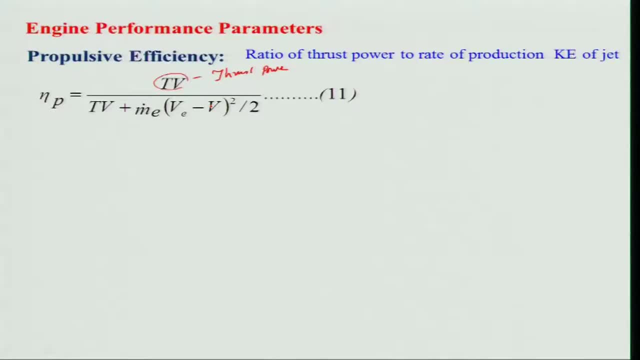 is being what you call being going out. you know, mass into this change in kinetic energy is going out. So this, if you look at, we are looking at with reference to what? with reference to the earth. right, If you look at this, if I look at the earth, 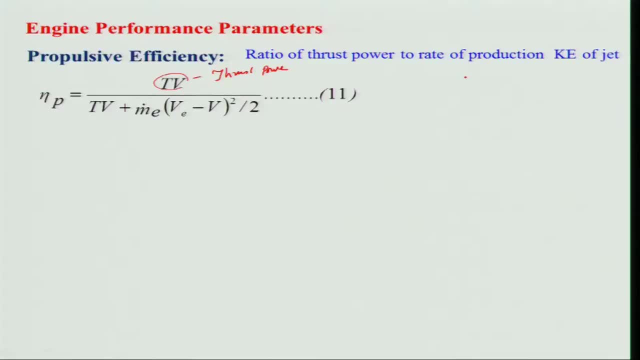 If you look at a kind of a vehicle, you know like that is a, this is a vehicle engine which is going this V e and it is entering with V right. So there is a person over here right. and with reference to that, how much V e changing this mass? you know it will be changing m dot. 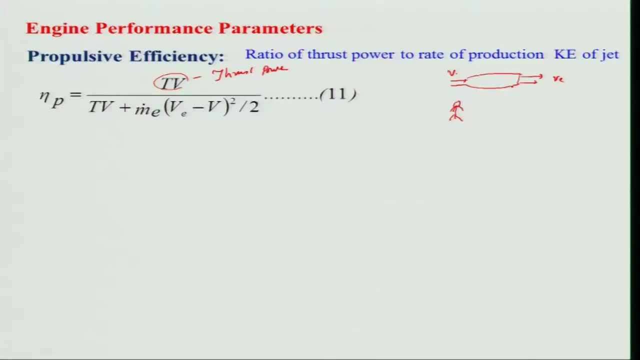 V e minus V whole square right. that is the mass which will be changing. So from my VSM, what we have looked at, that is m dot a 1 plus F, V e minus V plus P e minus. 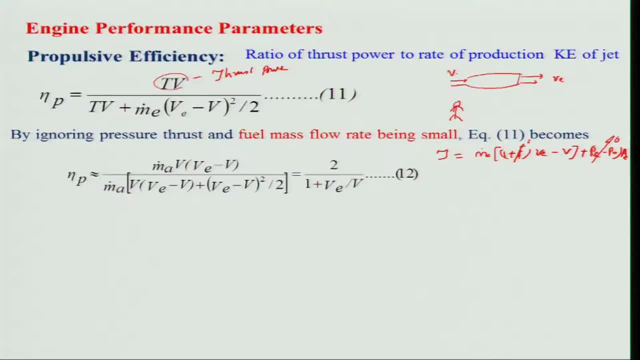 P a into A e. right, We are saying this is 0 and this is also 0 f. It is not true. but we are saying, for the simplicity, then I will get m dot a V e minus. this will be equal to m dot a V e minus P e. 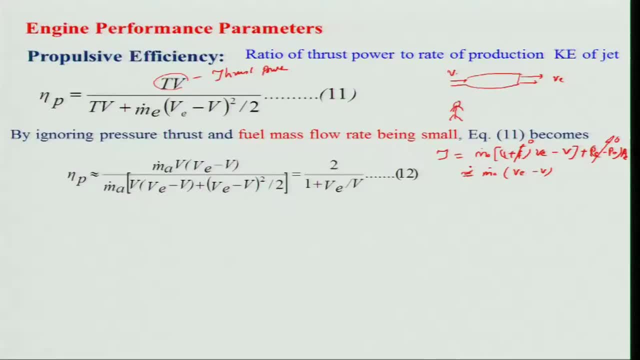 minus v. Actually, this is approximately equal, and this is my thrust, and v is the velocity, that is the power, and then m dot a and I will be using the same thing: v, v minus c, and this is the whole square, because I have taken in place of m dot e, I am using basically m dot. 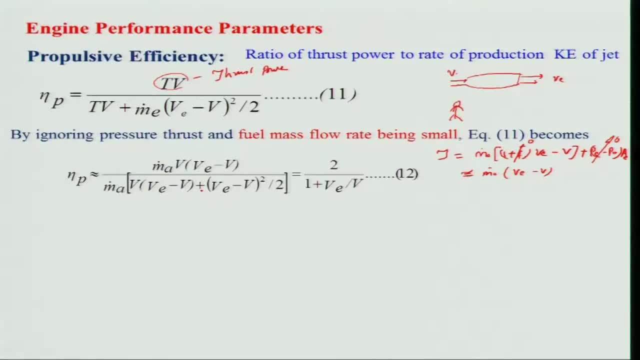 a. So I will take it out. and if I simplify this thing, you know, if I take v e minus v out of this place what I will get. I will take this v e minus v, So this will cancel it out, and this become v e plus v e minus v divided by 2. and if you just simplify that, 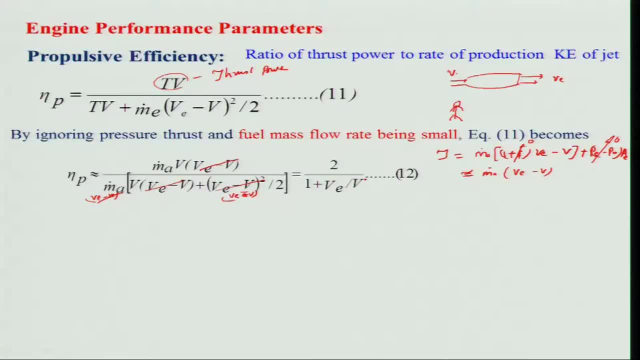 you will get basically 2 plus v e divided by v. What is indicating? It is indicating that the propulsive efficiency will be dependent on the exit velocity and flight velocity ratio, and when it will be 100 percent, When v e is equal to v, that means exit velocity is equal to the flight velocity. n p will be 1. that means 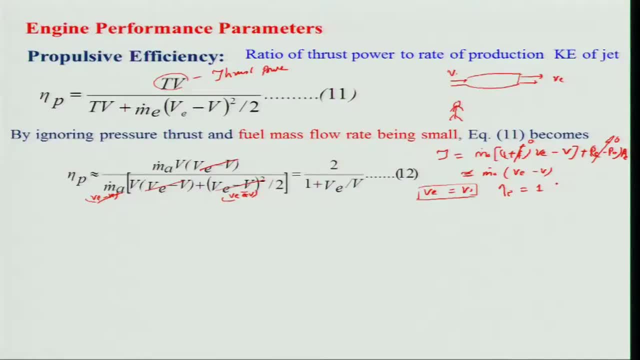 100 percent propulsive, is it quite a great, you know, is it possible? we can get that. So now for the rocket engine or the non air breathing engine, equation eleven. we can have right, we can get the similar way, that is, m dot e v into v? e. because in the rocket engine, what we are saying, We are saying: 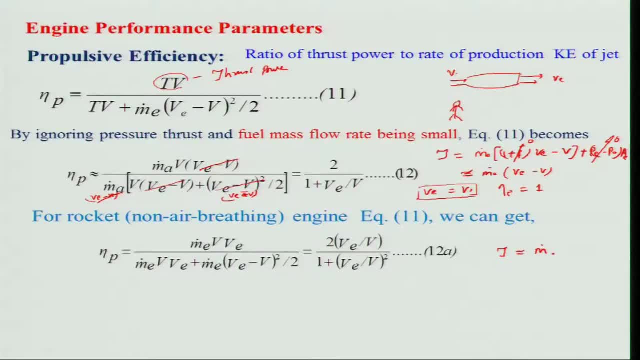 that m dot approximately equal to m dot v e, because is a fully expanded nozzle. we are assuming p e is equal to p a and there is no v right flight. If you look at, no air is into engine. So my thrust expression will be m dot, simply v? e. So I am putting it here. 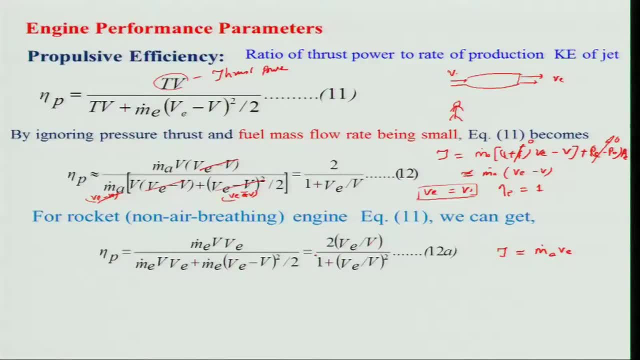 and if I simplify, I will get 2 v e divided by v, divided by 1 plus v by v whole square. You look at it is similar but not same. that is the difference. that is, this is a square is coming in the 1 plus v e by v square. and here there is another term: is coming on the. 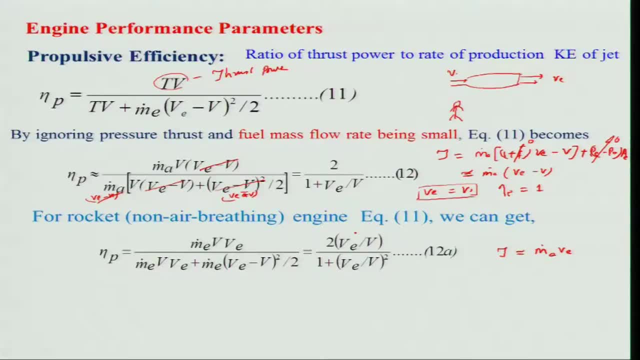 numerator. So that is the difference. and in this case, if I want to find out when it will be, the propulsive efficiency will be maximum, that will be again v. e is equal to v, am I right? Because if I say this is 1 and this is 1, 2 by 2 it become 1, 1 means 100. 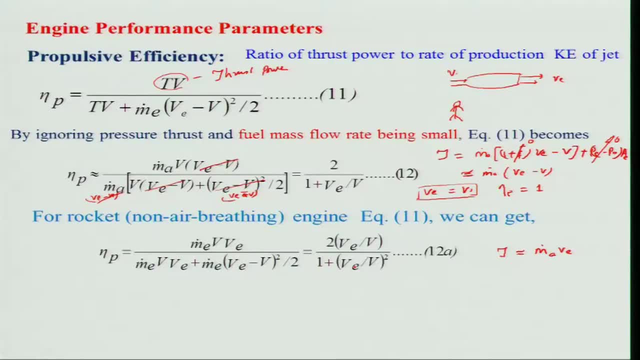 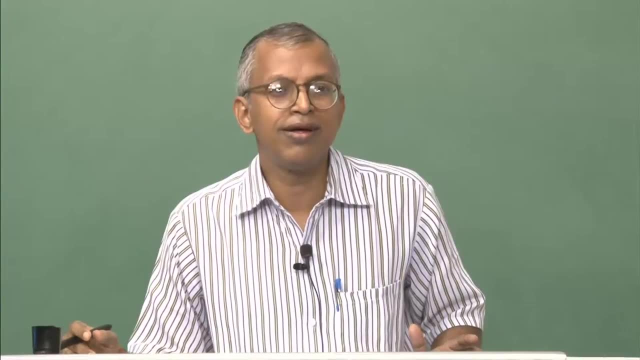 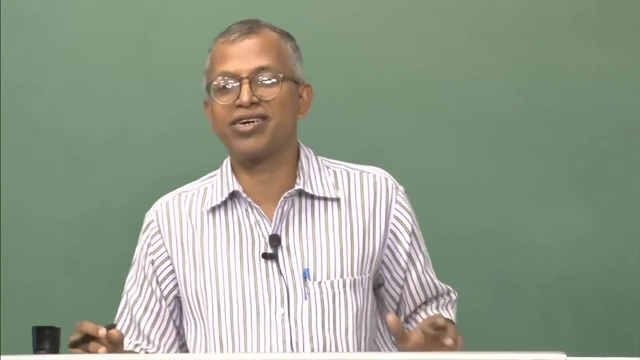 percent more than that. you cannot, because how much energy you are giving, you are all getting back in the or converting into thrust power. So is it really possible? that means whatever energy I am giving, I am just taking, I am just utilizing it to converting. If you can do that, that will be wonderful. I have already 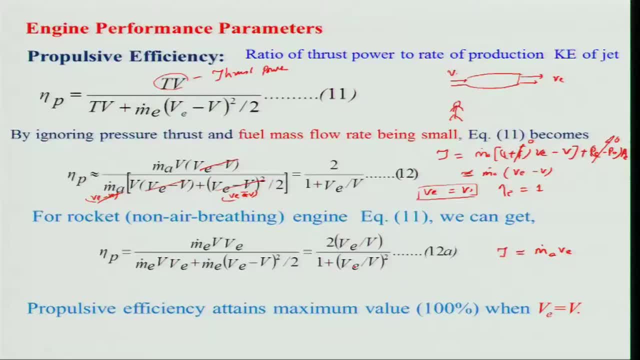 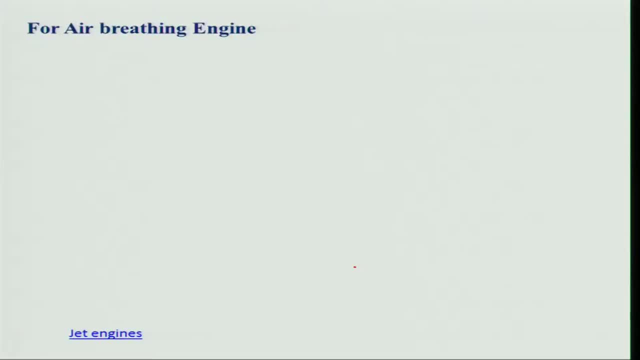 discussed that you will get maximum propulsive efficiency when v? e is equal to v. exit velocity is equal to the flight velocity. Now let us look at for air breathing engine and little bit talk about the efficiency. what is happening, ства isimenti how it is changing with the velocity ratio, that is, exit velocity and flight velocity. 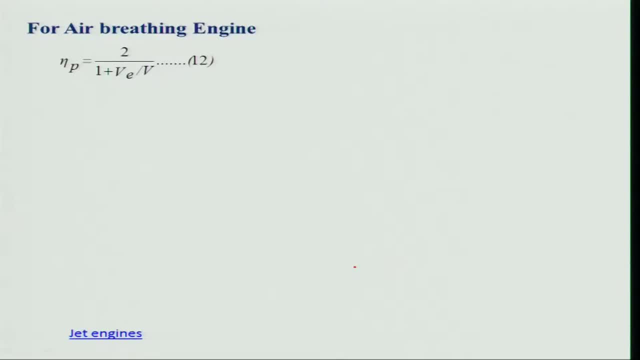 ratio. Exit means exit from the engine and flight velocity, of course, in this case in the air breathing engine, the velocity with which air is entering into the engine. So if you look at, if I look at, this propulsive efficiency, the v you will find at when v. 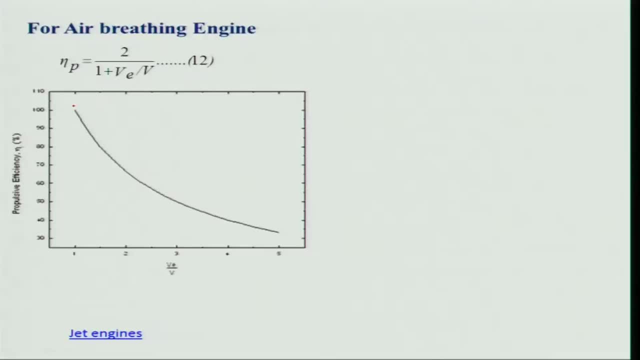 e is equal to v 1, same, you are getting 100 percent after that. it is decreasing. That means when the exit velocity will be go on increasing for a particular flight velocity, what will happen? Propulsive efficiency decreasing. That means if I want to fly, an air breathing 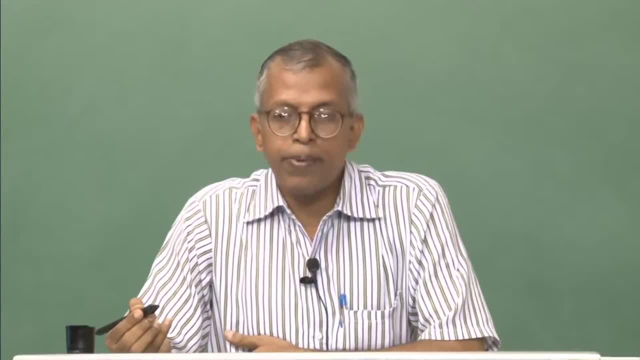 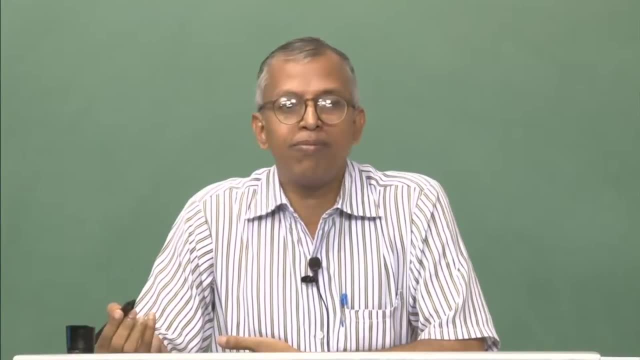 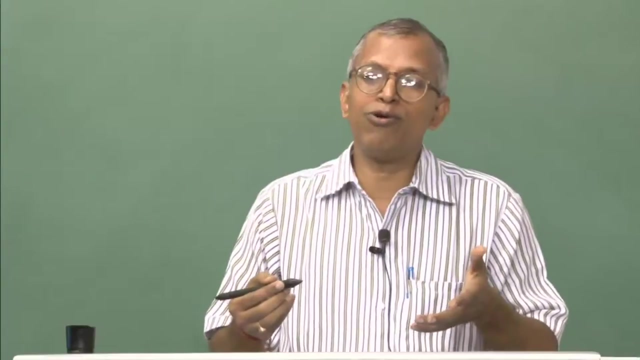 engine for a particular flight velocity. that means, if I want to fly an air breathing engine, then if I go on increasing v I am in trouble because the propulsive efficiency is coming down. But if I want to, always we want to maximize the propulsive efficiency, am I right? 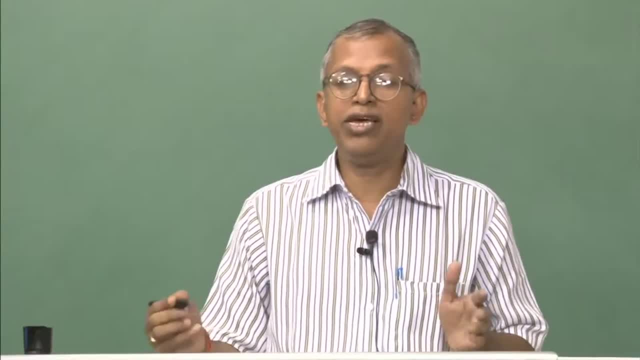 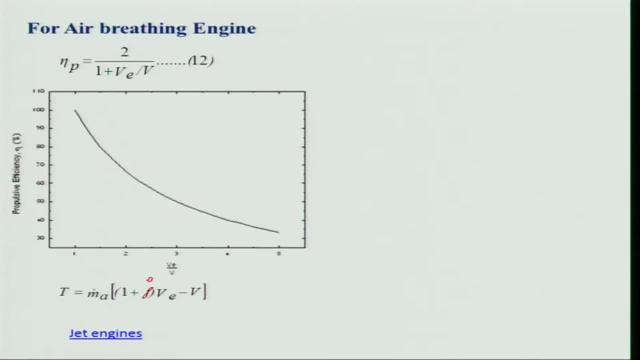 But if I maximize what happens, If v, e is equal to v, then what happens? Thrust will be 0.. If I say this is, you know, 0, so or approximately 0, or in a compared to, so I can say that thrust. 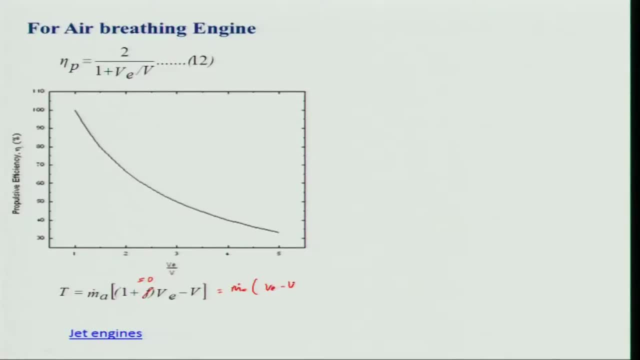 will be 0.. M dot a v e minus v is equal to 0. for v e is equal to v, but propulsive efficiency will be 100 percent. for this condition That means I am having trouble If I go one extreme side. 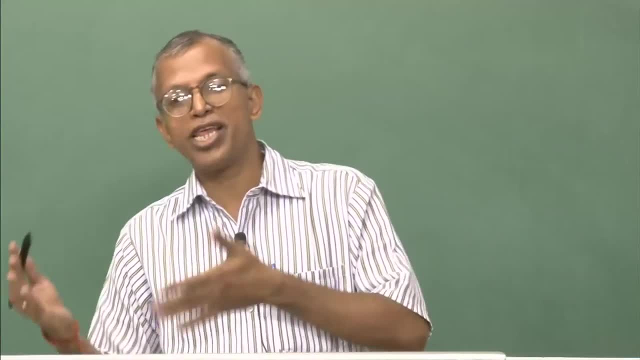 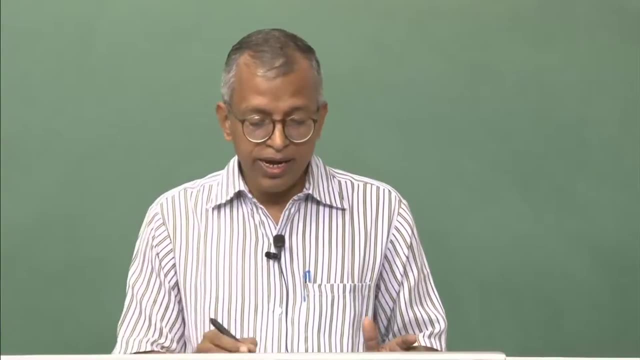 I am getting 100 percent efficiency, thrust is 0.. If I go other way around, that is, you know, v e is far greater than the v, Right, I may get higher thrust If v e is greater than v, far, far better. you know like. 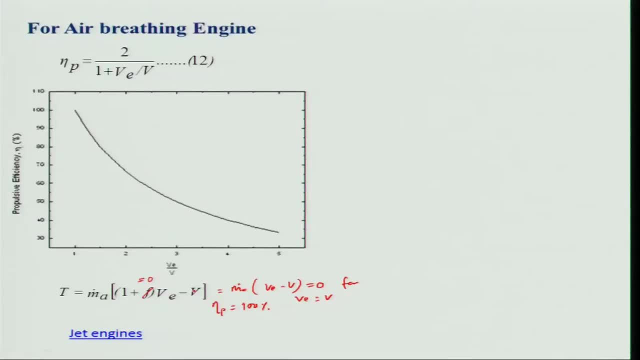 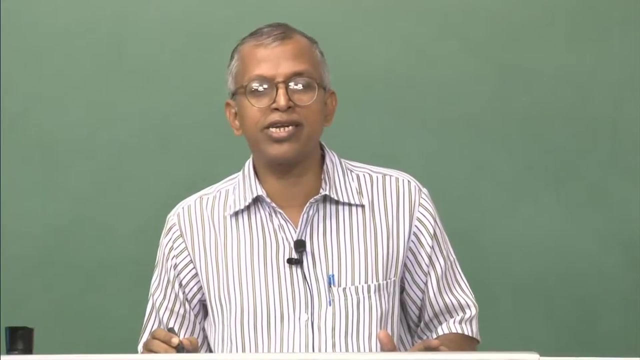 v can be negligibly small flight velocity, then I am getting the maximum thrust right, But my propulsion, what I will do, It is like that, what I started this talk like. if you have too materialistic, or what I call, you know stinkingly materialistic, then you 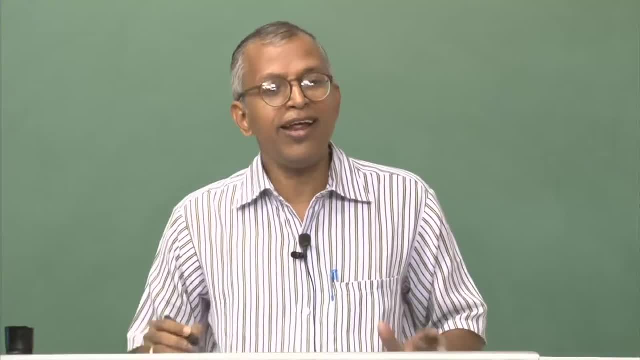 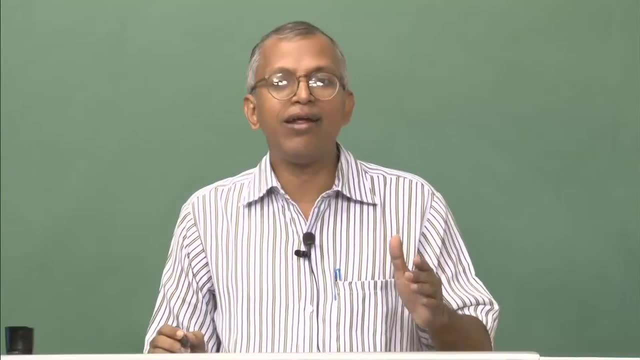 will be in deep trouble. That what we are today. and if you say that I do not want materialistic, realistic, then you cannot survive. So you will have to take a middle path and based on these things, there are several kinds of engine. people have developed jet engines. 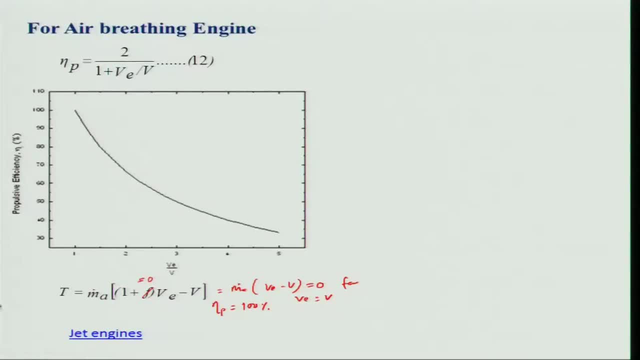 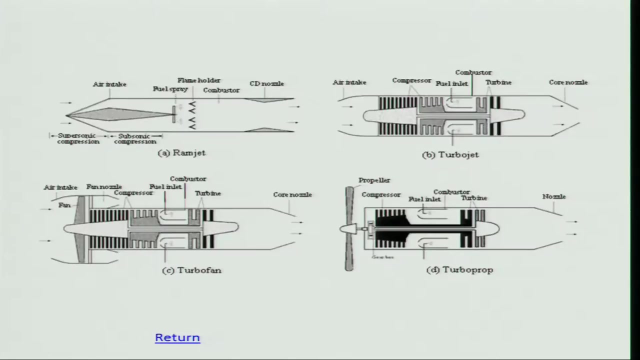 What are those? That is, basically, what are the jet engines you know, based on this concept, What are the engines? you are aware? That is ramjet, turbojet, turbofan and turboprop. So if you look at I have shown you schematically. we will be again visiting. I am not. 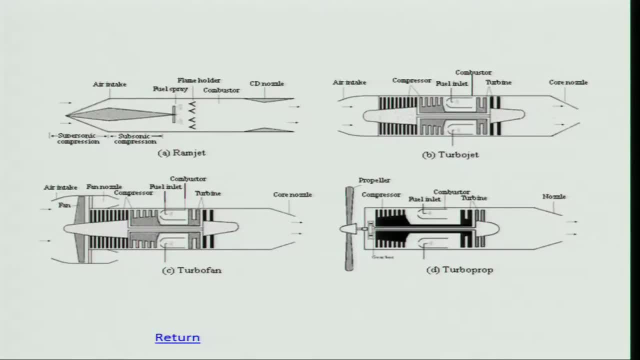 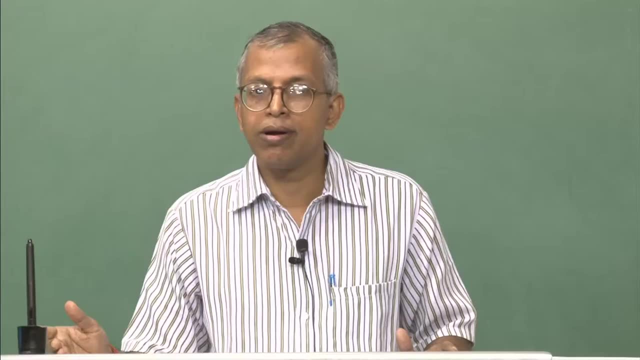 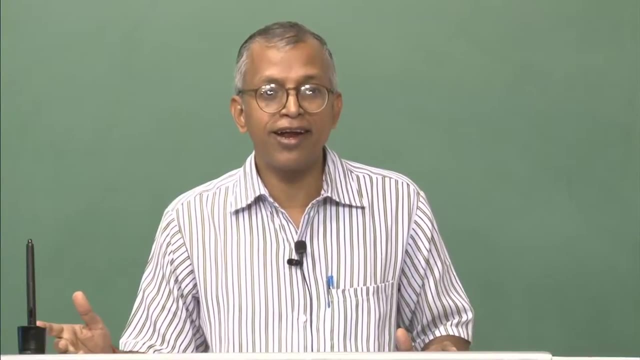 really discussing about that. but what really is happening in the ramjet? Ramjet will be flying at a very what High Mach number, and what happens to exit velocity? It is also equally high, right? That means in this case what I will get My propulsive efficiency. 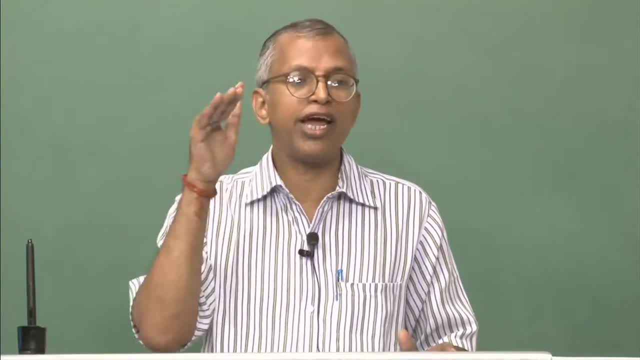 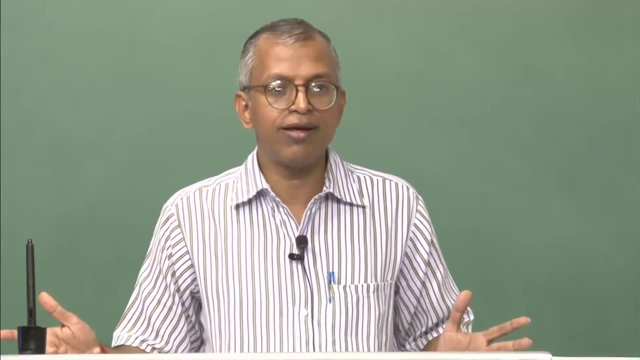 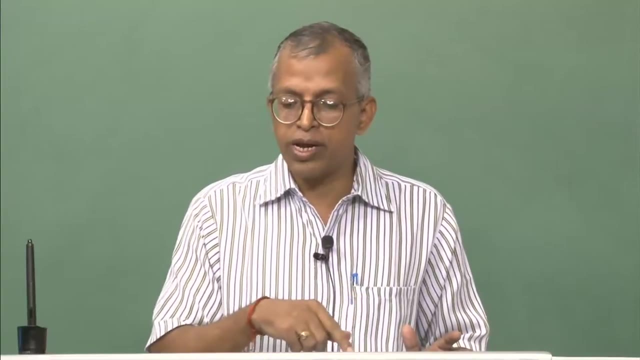 will be very low, because if I want to fly at a high Mach number, then naturally I will have to give a higher thrust, Otherwise I cannot. Can I For the same kind of drag? you know like I cannot. So therefore, here, propulsive efficiency is very low. and as you go on to, 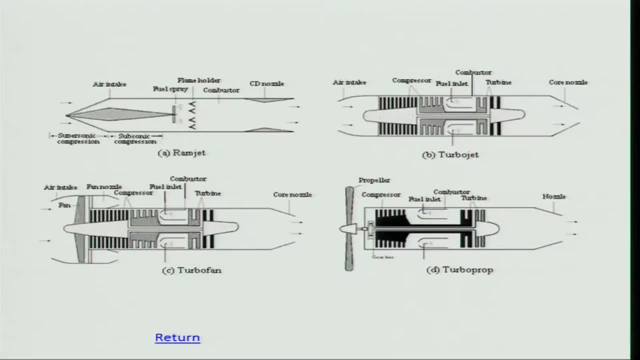 turbojet. it is, you know, propulsive efficiency: lower than the, you know, higher than the ramjet, but thrust will be lower than the ramjet and turbofan thrust will be lower than the ramjet. So these are, you know, medium kind of thing, propulsive efficiency. 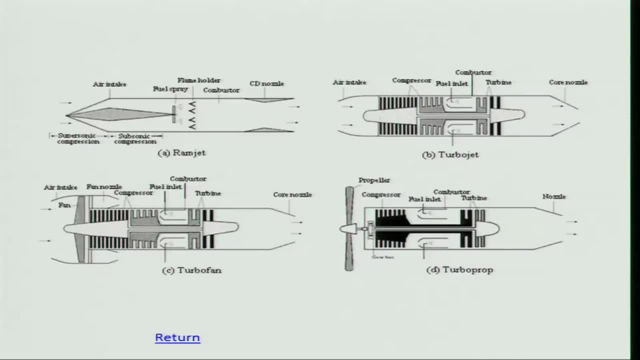 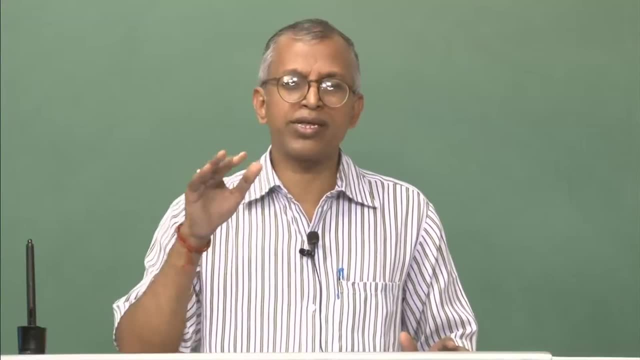 will be quite, and if you go to turboprop, propulsive efficiency is the highest but the thrust will be very, very low. So you will be at a slow moving or something. we use a turboprop engine right. So we will be discussing about that, but let us look. 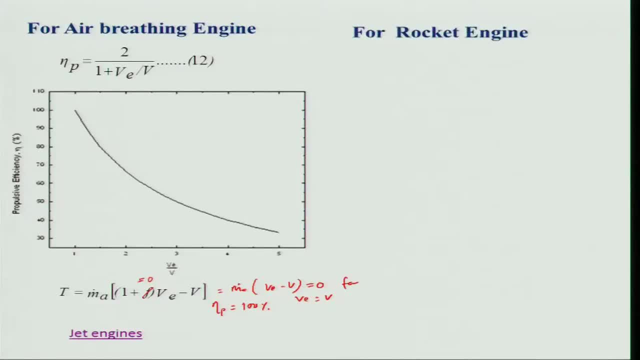 at now, the rocket engines, right, How, this propulsive efficiency varying with the V, e by v, how it will be, Why it is How it will be. You know you are trying to find out what, right, How this? you know what you are trying to do. What do you know How this AC of right? 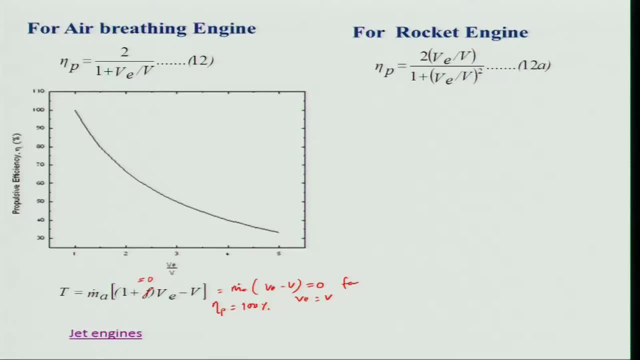 it will be varying. Will it be varying the similar way that is goes on decreasing? Certainly no. If you look at this expression, you will find that propulsive efficiency is increasing. you know from the 0, because I can have you know, v, e or v may be very high as compared. 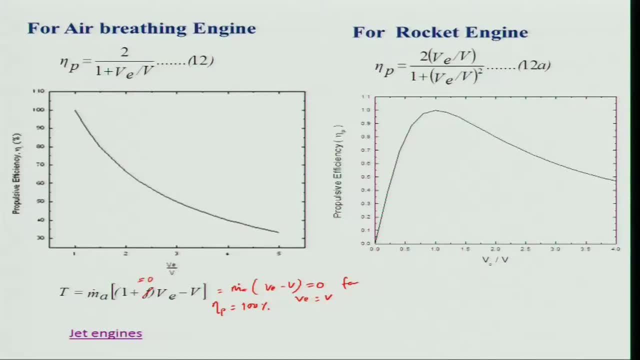 to v e. That means I am going towards 0, but in reality is not possible. So it will be, of course, from this expression is being plotted here, So it will be. goes on increasing till it reaches v. e is equal to v, you know. the velocity ratio becomes 1 and after that it 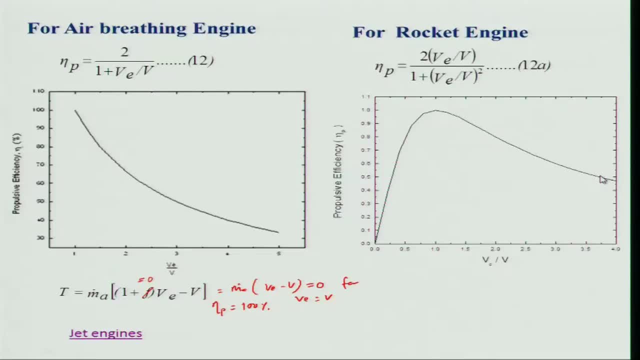 decreases. Generally it is not possible to maintain this. v e by v is equal to 1, because it will be all accelerating. So therefore people try to operate in this regime where propulsive efficiency will be very high. So this is the reason people do not operate, although sometimes during the static, you know. 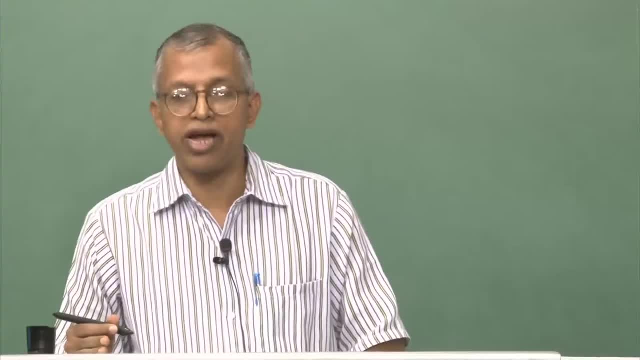 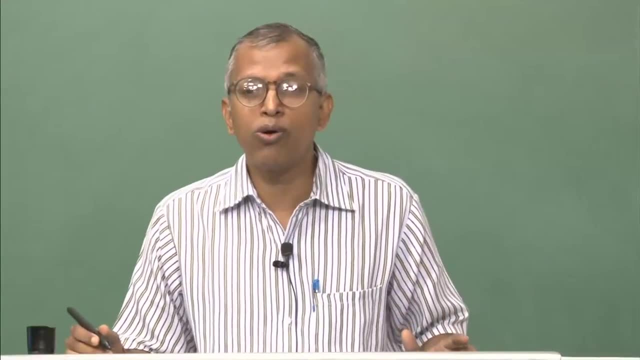 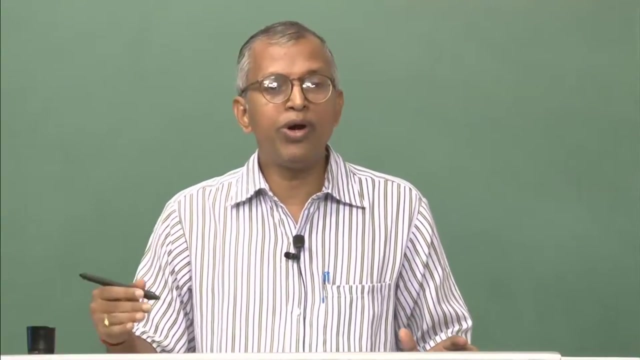 during the intake may be sometimes, but that is a very small time. Now we will be looking at thermal efficiency, because this is about propulsive efficiency, which tell you how good your engine is giving, providing the what you call thrust power. but now we need to look. 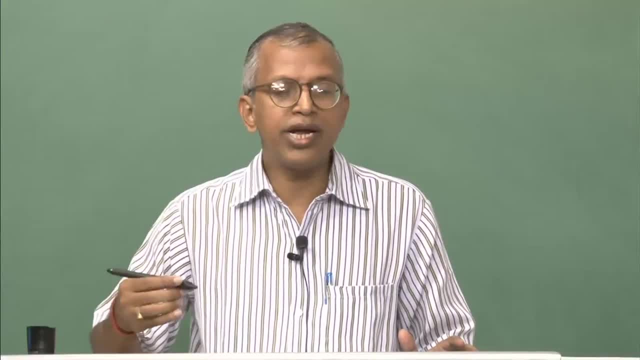 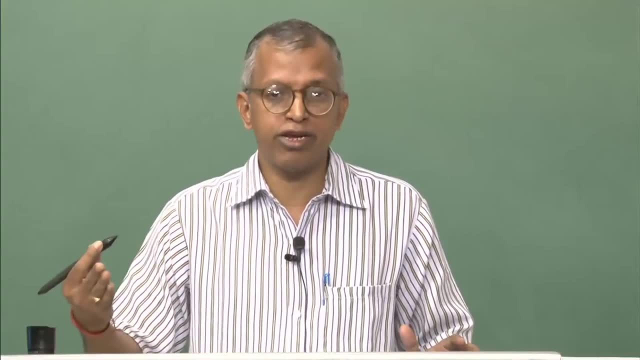 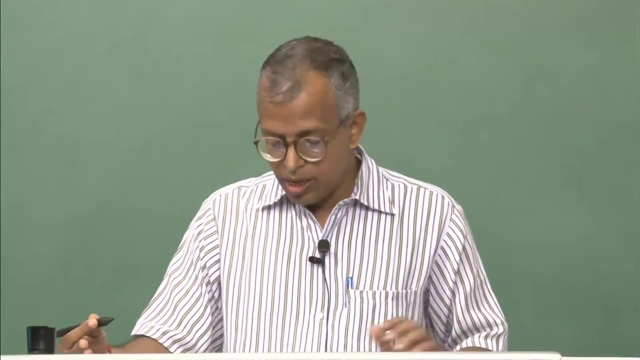 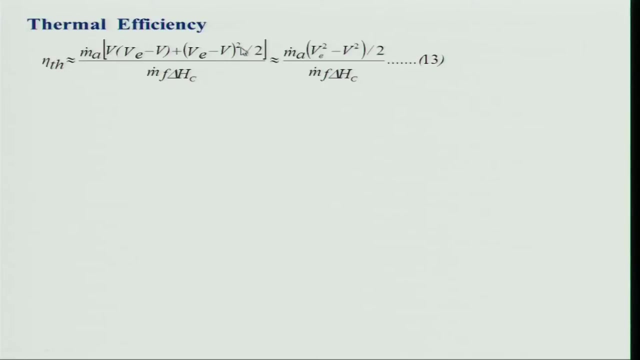 at right how good it is in converting the fuel iggly are the, you know, chemical energy into the kinetic energy. because here what we are using change in kinetic energy, We are using to get the thrust power right. So that means this is: we can say that the thermal efficiency is a ratio of the kinetic energy into the 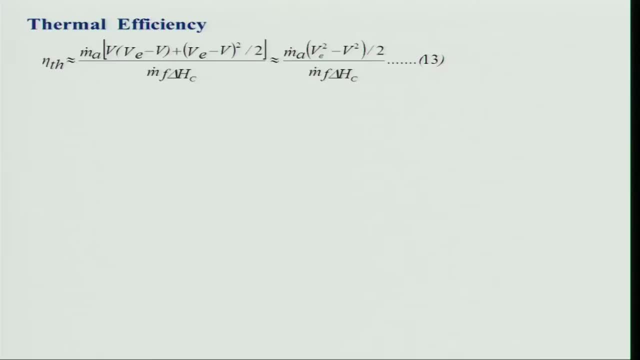 amount of energy or the fuel being burned. That means total chemical energy. if I just simple this and then if I expand this one, you will get that is equal to m dot, a, v, e minus v, 2, whole square. This is nothing but your kinetic energy. change in kinetic energy divided by: 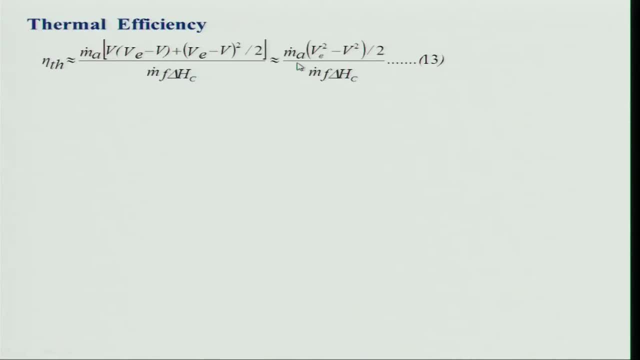 m, dot, f, delta, s, c. So keep in mind that here what are the assumption we are doing? because I am not using same as equal, because the same assumption we are doing, the nozzle is fully expanded. that means there is no pressure. you know, thrust from the pressure, different change. 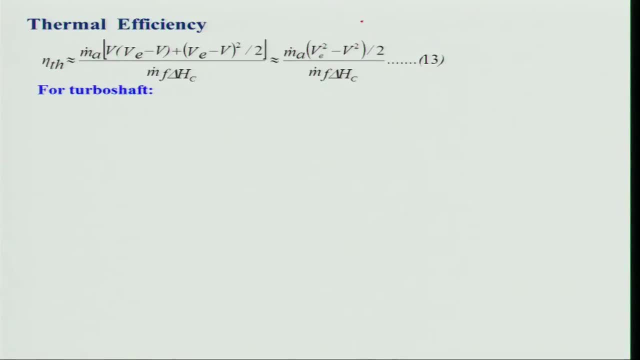 and also the m dot f is very much less than the m dot a, or f is less than 1.. So that assumption we have made. but however you know, for the turbo shaft engine, you know we cannot really talk about that kind of thing because the flight velocity would not be there. So 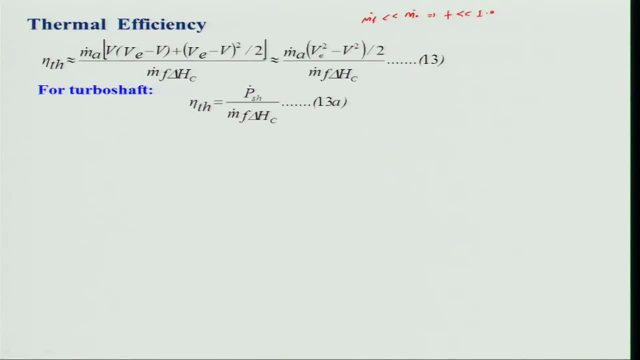 what we will be looking at. We will be looking at the, instead of change in kinetic energy, we will be looking at the shaft power, because in the turbo shaft engine, you know we use the shaft power, So therefore I can use p, that this is basically shaft power, and m dot f, delta s, c. m dot f is the fuel. 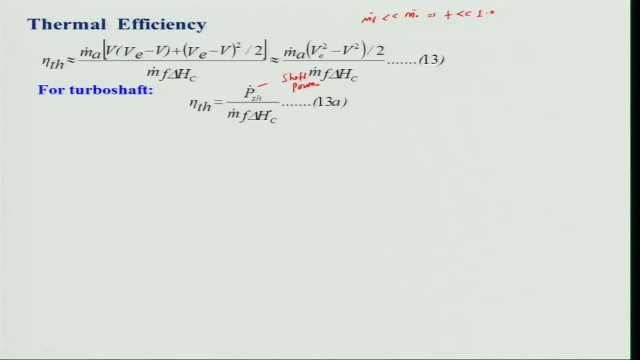 you know, consumption rate into s. c is the heat of combustion, and keep in mind that we are assuming the combustion efficiency is 1.. This is the one which we are not considering in this case, but in real situation it would not be. So now, overall efficiency will be what Overall efficiency will be basically. 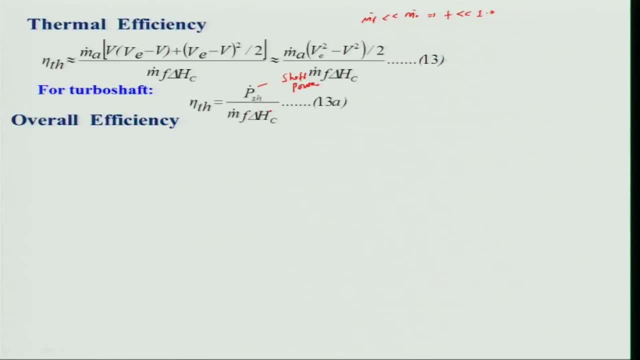 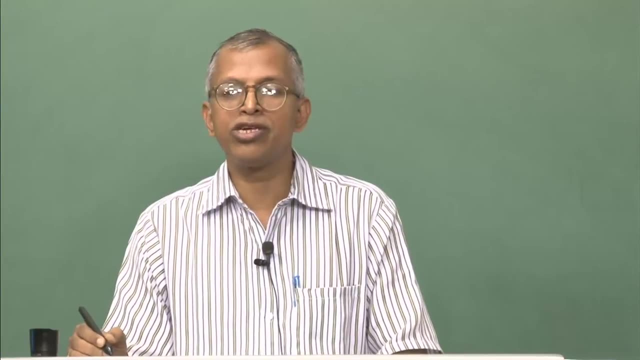 the populsive efficiency and the thermal efficiency. in other words, it will be the thrust power, ratio of the thrust power and the amount of energy being consumed or being, you know like, used for that. So the other one is the thrust power and this is the number of energy which 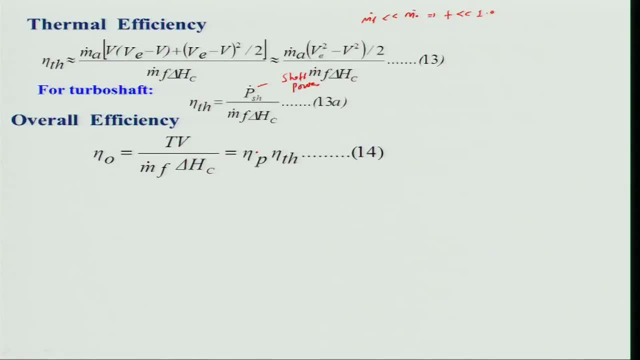 is consumed at this level. Now, if the thrust element is FEMA in this form, that means you know it is consumed currently. How can you get the current energy which is consumed at this delta s, c? and you will find that you can derive this. I mean, which is very obvious, that 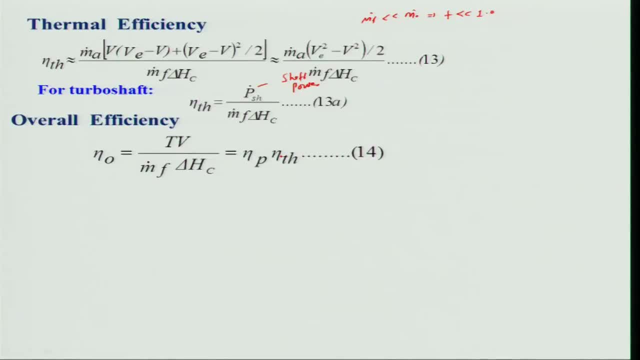 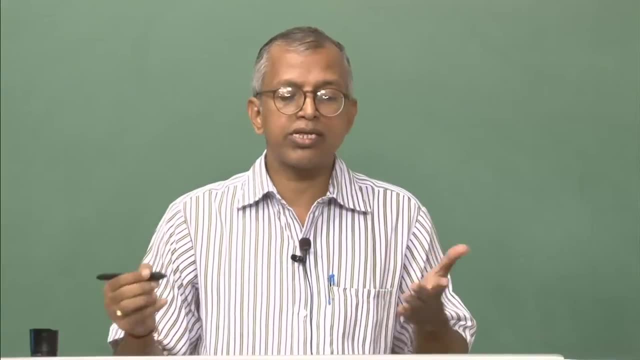 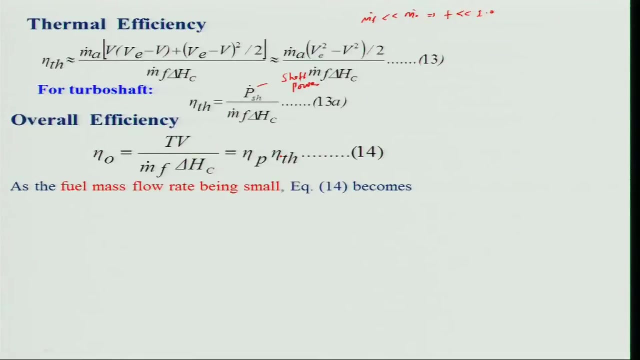 propulsive efficiency into thermal efficiency. Now question arises how it will be varying this overall efficiency with respect to, let us say, velocity or velocity ratio. So what we will do, We will again assume the same assumption, that f is very small, or the fuel. 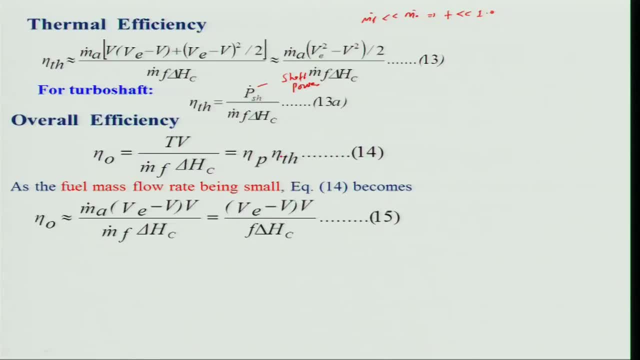 mass flow rate being small. So equation 14 becomes- you know like this what I am doing: m dot a, v e minus v. I am using the thrust and I will find out v e minus v into v, f, delta, s, c. And if you look at for a particular fuel, air ratio or a particular kind of fuel, you 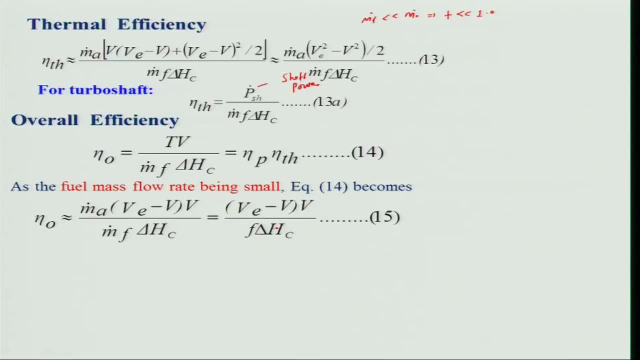 will find that it is dependent on the v, e and v, That is, exit velocity and flight velocity. And what we will do. We want to find out what is the overall efficiency of a propulsive device or the engine That is more important. 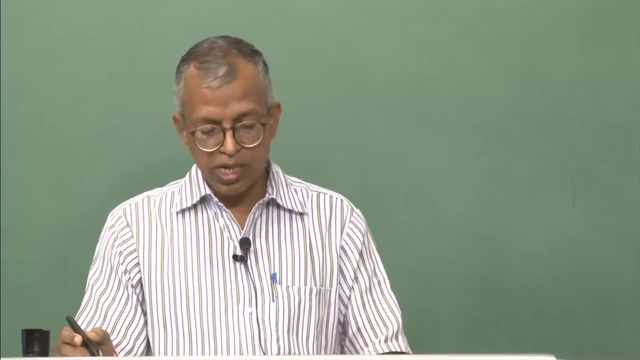 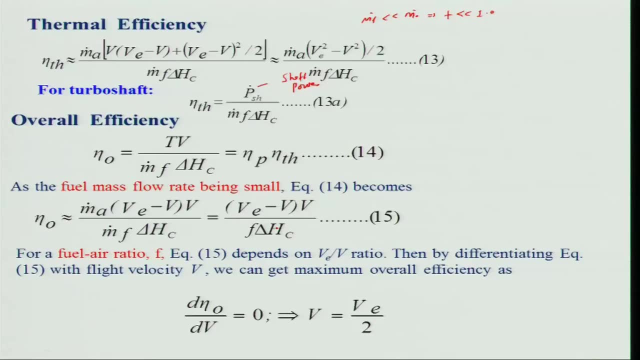 than that of propulsive, only propulsive efficiency, thermal efficiency. So for that what we will do, We will differentiate this equation with respect to v, the flight velocity, And we will find that is equal to 0. So what we will get When the flight velocity is half of the exit velocity you will get: 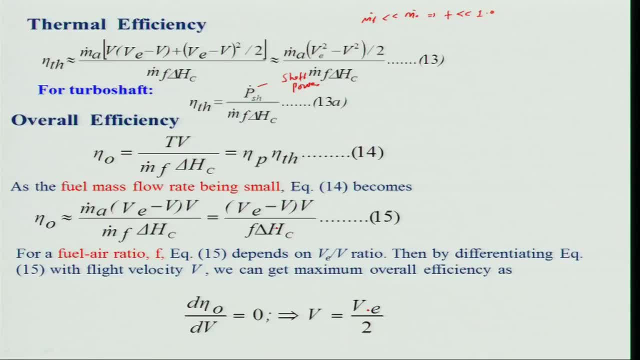 a overall high maximum overall efficiency, which is, you know, generally the case being used, particularly for your Boeing kind of series. And we will see also why this long range commercial, or the rather passenger aircrafts you know, is being operated at maximum speed. 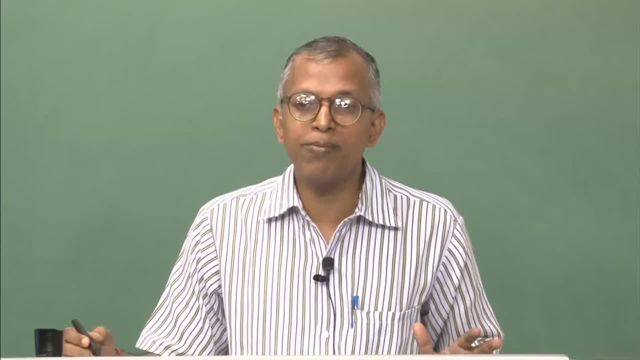 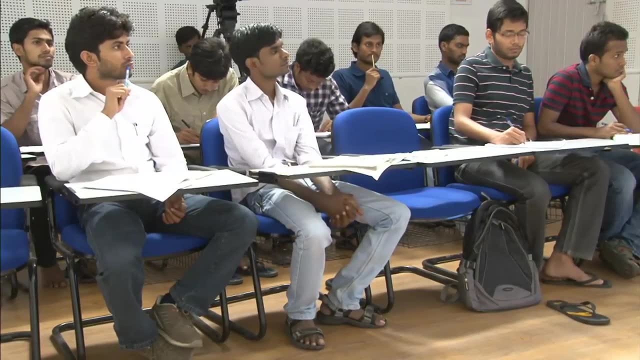 What is the maximum speed It is being operated at, Mach number of what? What is the Mach number it is being operated? 0. No, 0.85 kind of things, or 0.8 kind of things, Why it is so. 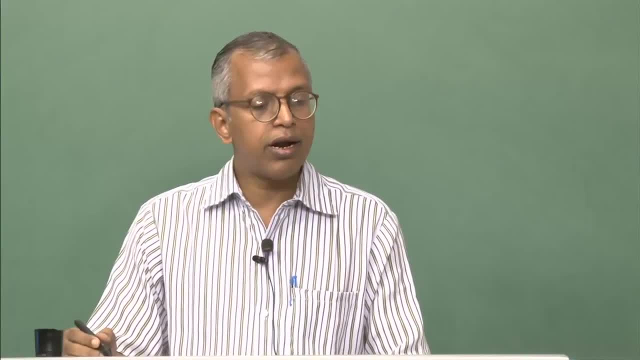 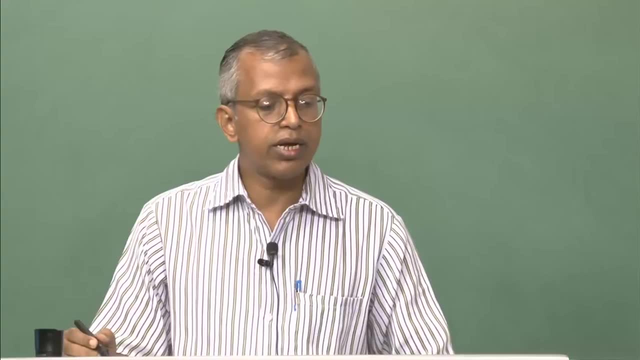 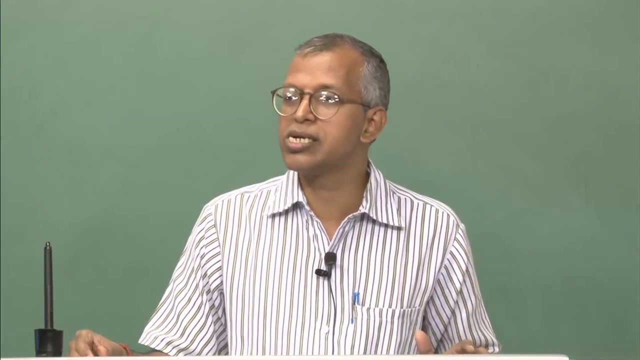 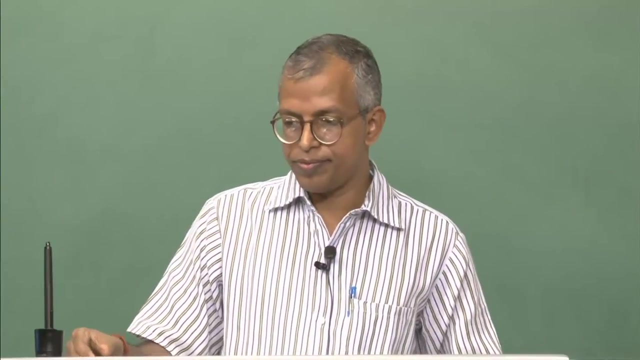 This is one of the reason, but another reason I can talk about it. I think I will stop over here and then we will discuss this thing in the next lecture And some of the more like performance parameter, like static thrust, Static thrust and other things And range, all those things we will be discussing. Thank you very much.